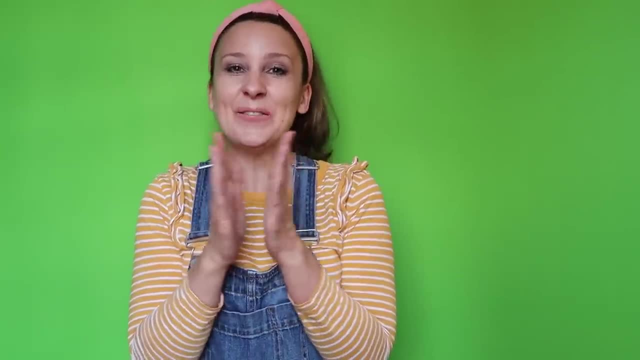 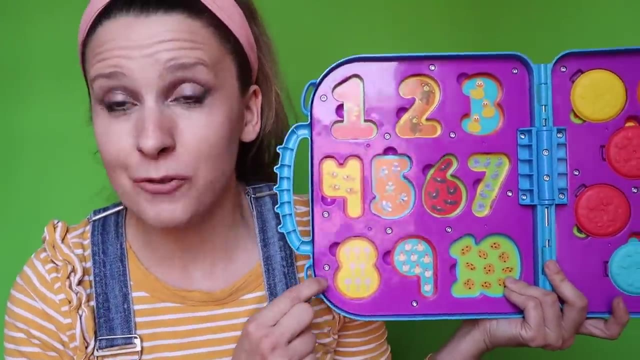 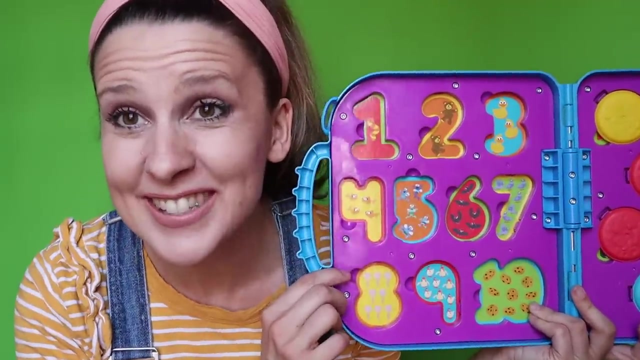 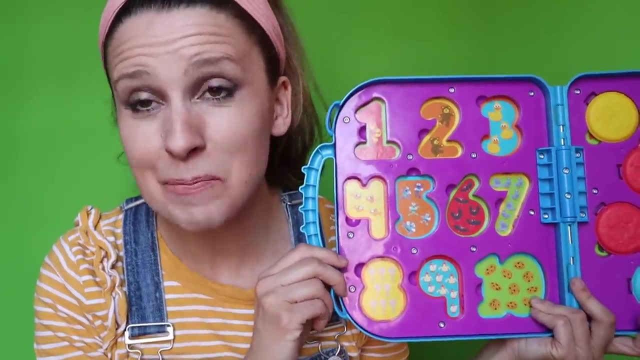 Can you clap? Great job. Oh no, All the numbers are missing from our number puzzle. Hmm, Maybe if we sing some songs about numbers, the numbers will come back. Can you help us sing some songs about numbers? You can? Okay, great, Thank you so much. Let's sing some number songs. 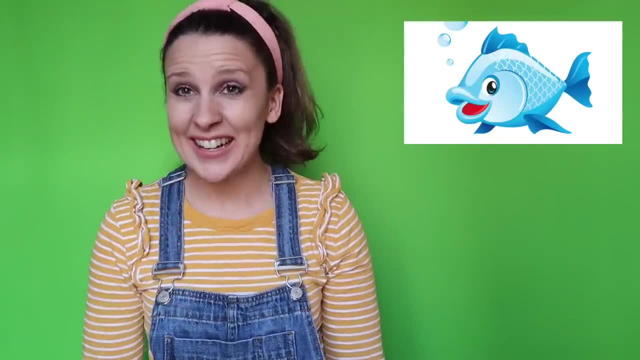 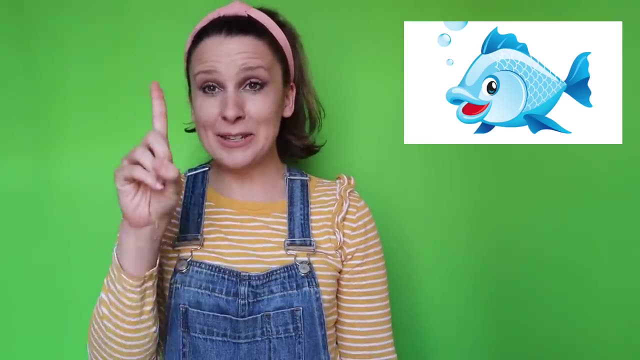 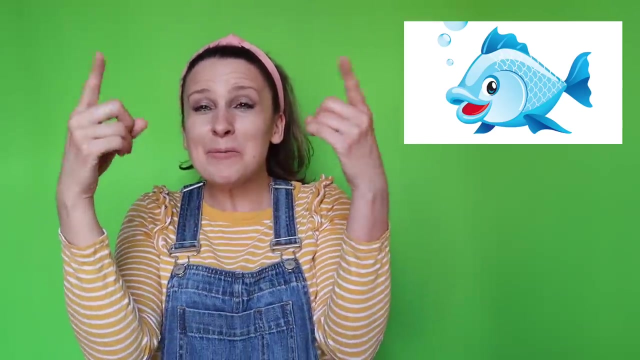 Let's get out one little blue fish. Are you ready? One little blue fish swimming in the water. One little blue fish swimming in the water. One little blue fish swimming in the water, Bubble, bubble, bubble, bubble pop. That was fun. Let's get out two little red fish. 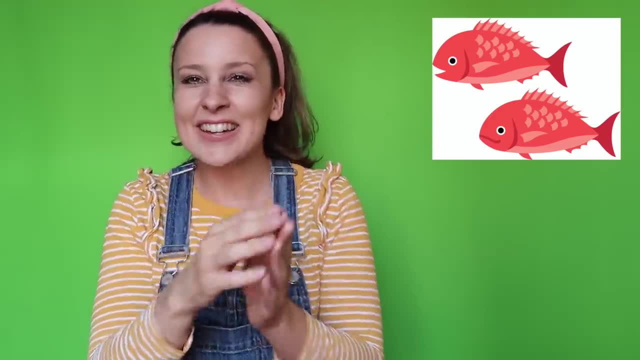 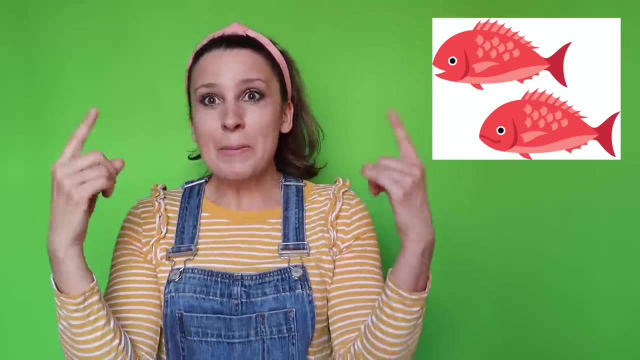 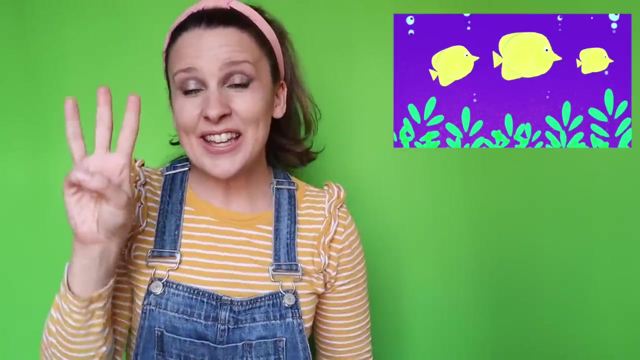 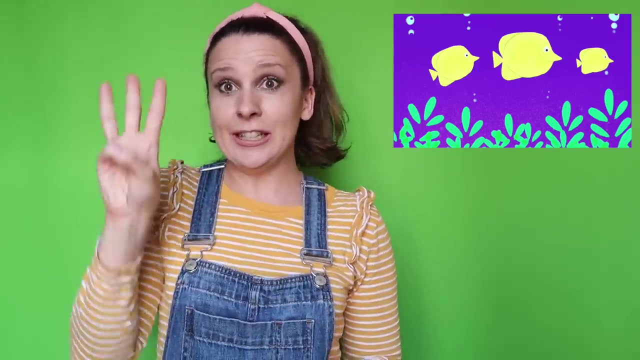 Two little red fish swimming in the water. Two little red fish swimming in the water. Two little red fish swimming in the water. Bubble, bubble, bubble, bubble pop. Wow, Let's get three yellow fish. Three little yellow fish swimming in the water. Three little yellow fish swimming in the water. Three little yellow fish swimming in the water. Bubble, bubble, bubble, bubble pop. 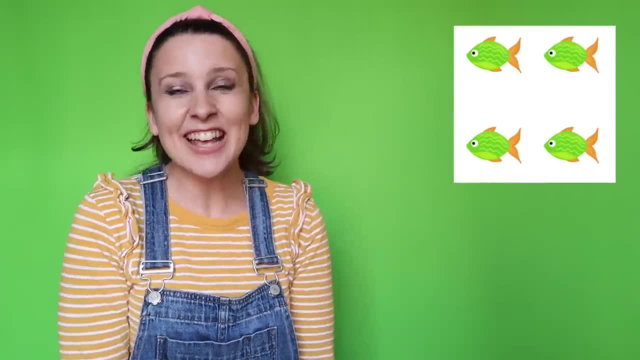 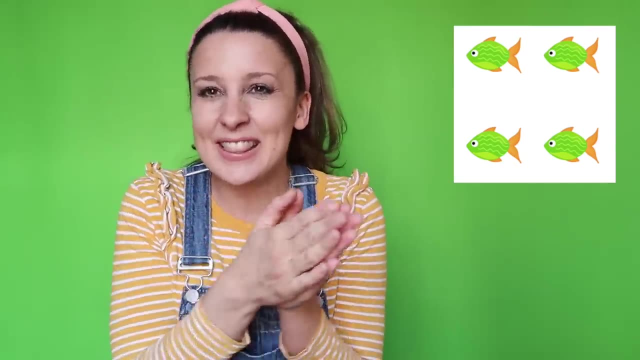 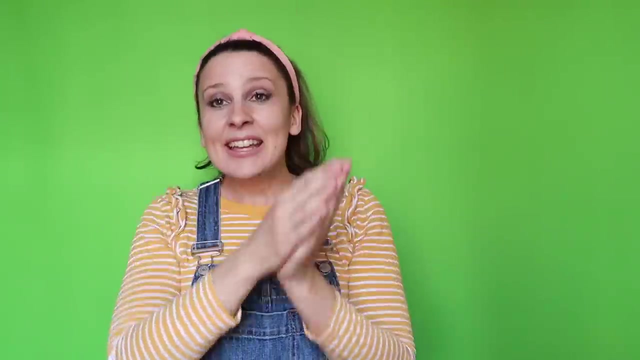 How about four green fish? I'm excited. Four little green fish swimming in the water. Four little green fish swimming in the water. Four little green fish swimming in the water, Bubble bubble, bubble, bubble pop. Now let's do five rainbow fish. 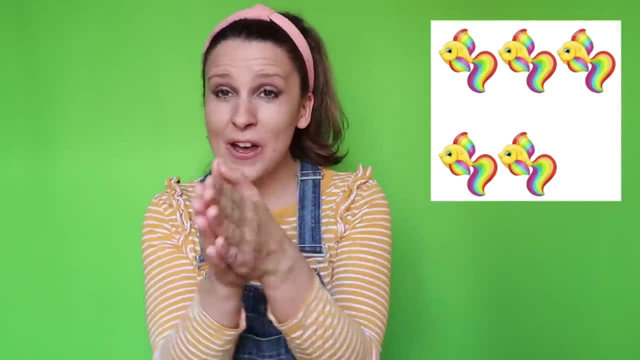 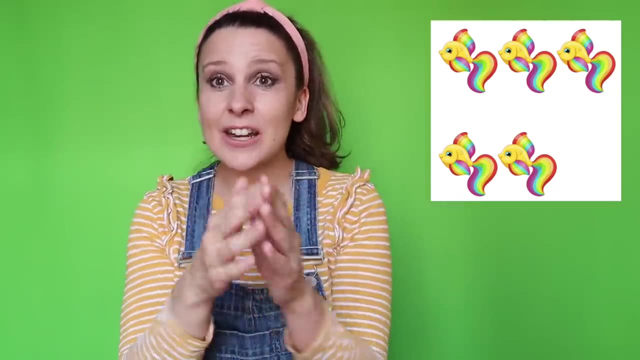 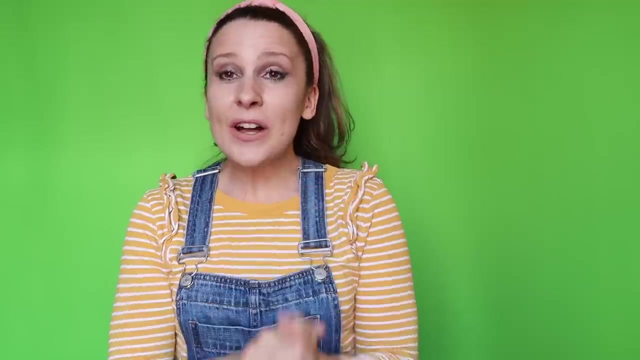 Five little rainbow fish swimming in the water. Five little rainbow fish swimming in the water. Five little rainbow fish swimming in the water. Bubble bubble, bubble, bubble pop. Wow, Great job. What color fish would you like to see? 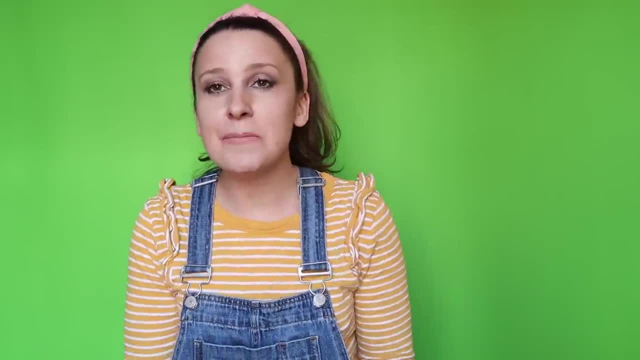 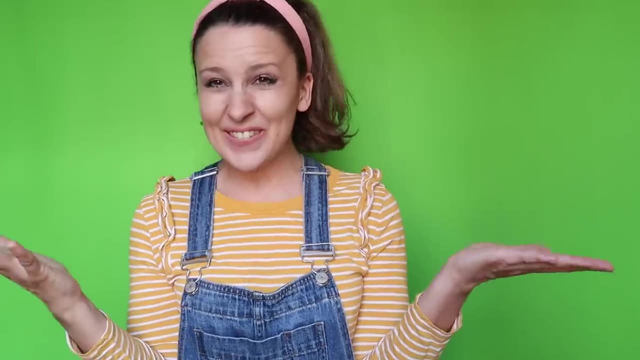 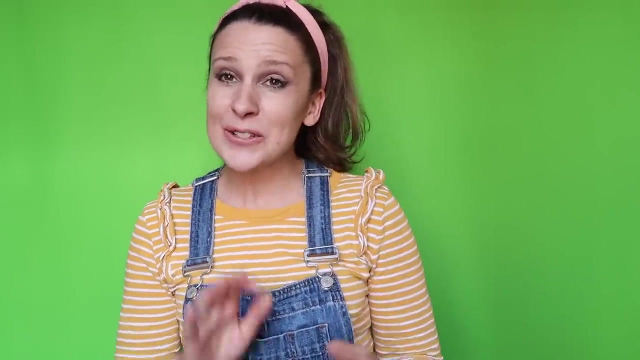 What color fish would you like to do? You could even do something like a Spider-Man fish, or a Batman fish, or an Elsa fish, or an Anna fish, or a really sparkly striped polka dot fish. I'd love to hear what you chose. Great job. 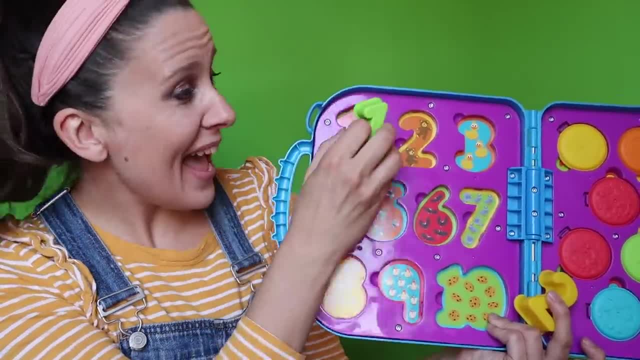 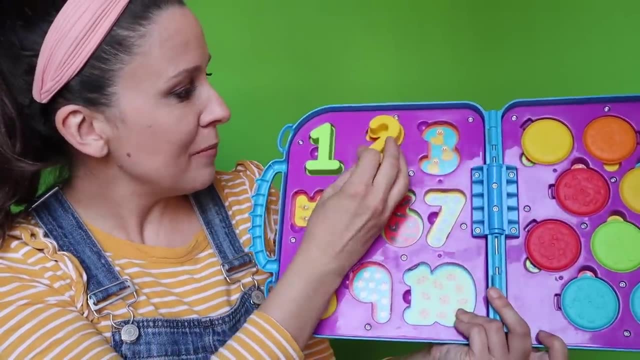 We sang a number song and number one came back. Yay, Let's put it in. And number two came back. Let's put in number two. Let's put in number two. Push, Number two is back. Let's sing more number songs, so more of the numbers come back. 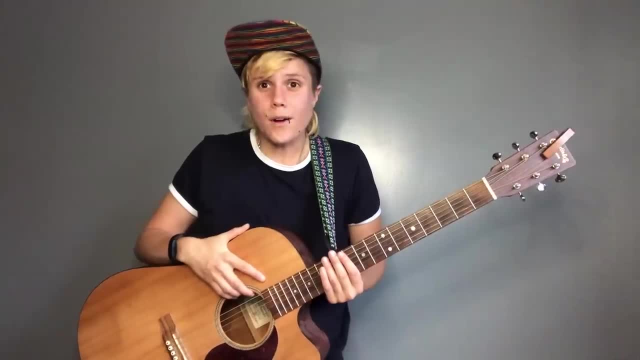 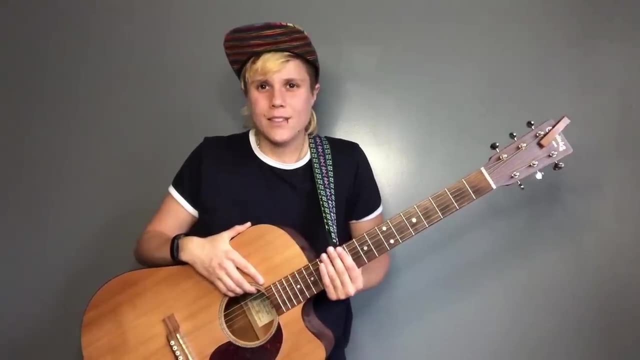 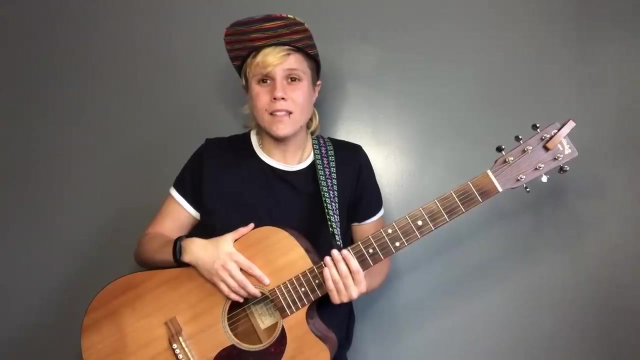 Hey everybody. it's Jules here. I heard you're learning about counting today. That is so cool. Counting is so important. Do you know how to count backwards? Hmm, Should we give it a try? Let's start at five and we're going to count backwards to one. 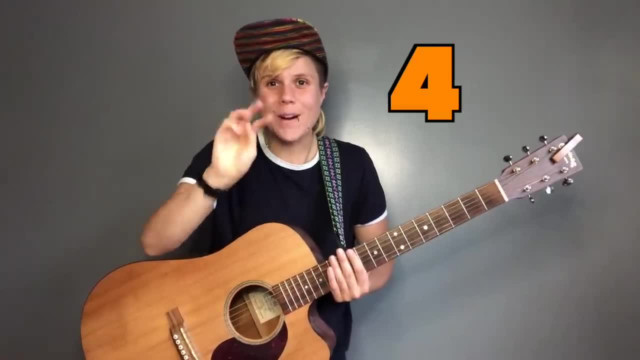 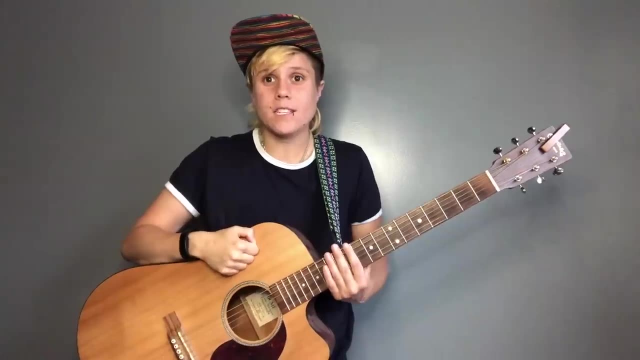 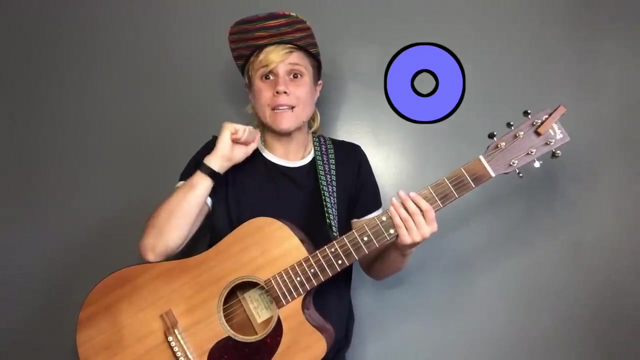 Ready? Five, four, three, two, one Today's song. we're going to count backwards. We're going to start with five green and speckled frogs and go all the way down to one or none. Are you ready? One, two, three, four, five green and speckled frogs. 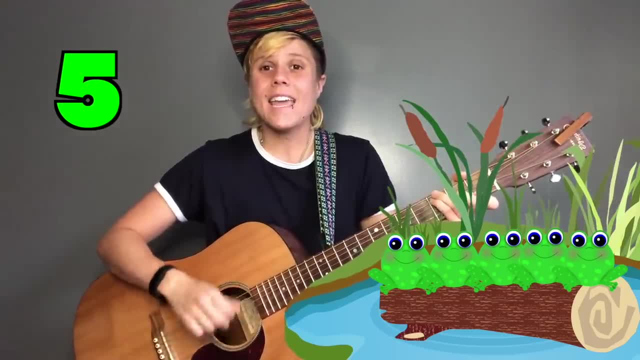 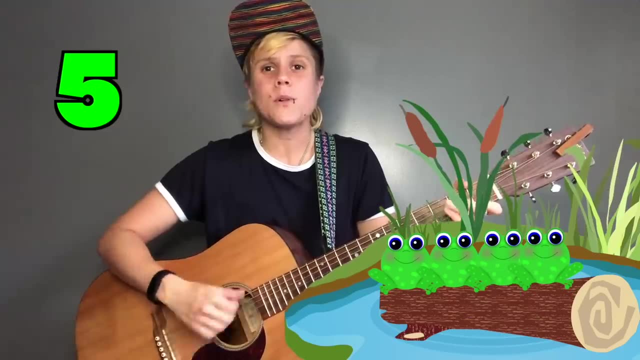 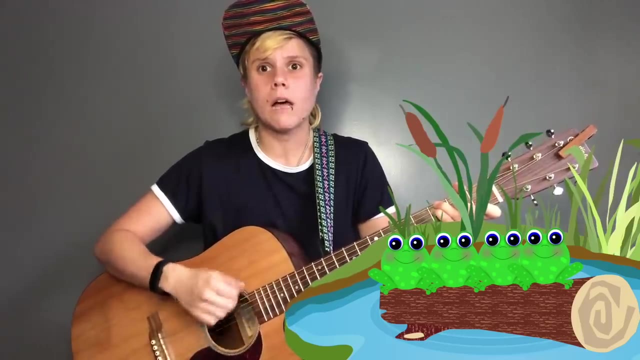 Set out a speckled log Eating some most delicious bugs. Yum yum. One jumped into the pool, where it was nice and cool. Now there are four green speckled frogs. Blah, blah, blah. Four green and speckled frogs. 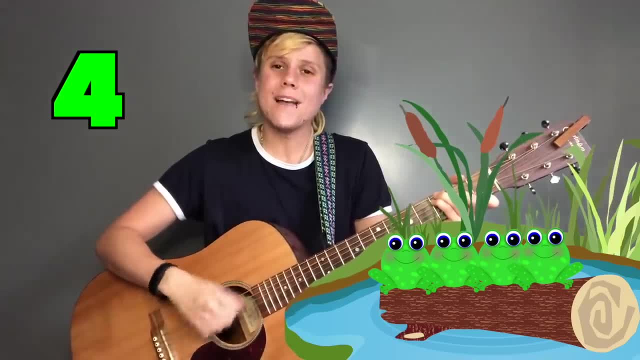 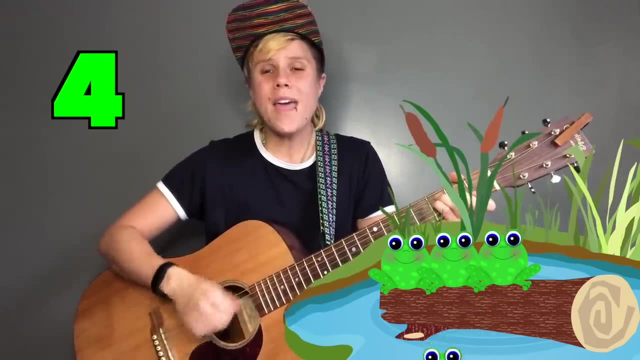 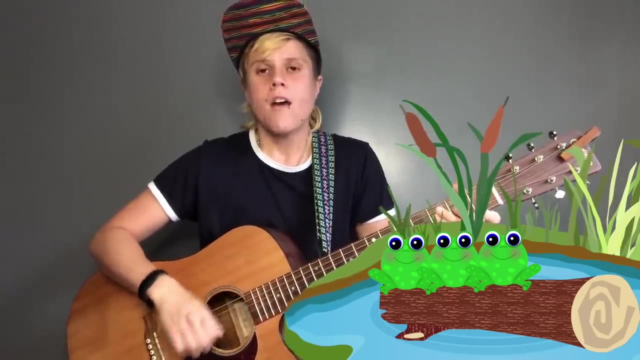 Set out a speckled log Eating some most delicious bugs. Yum yum. One jumped into the pool, where it was nice and cool. Now there are three green speckled frogs. Blah, blah, blah. Three green and speckled frogs. 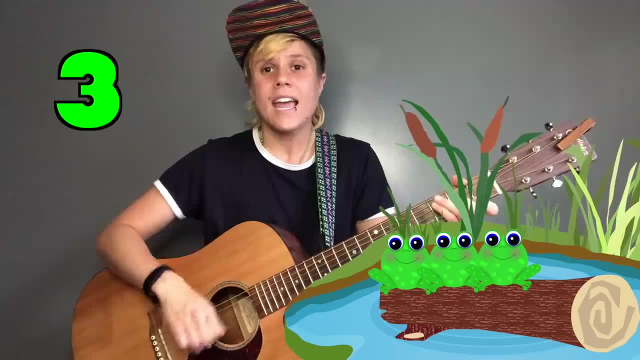 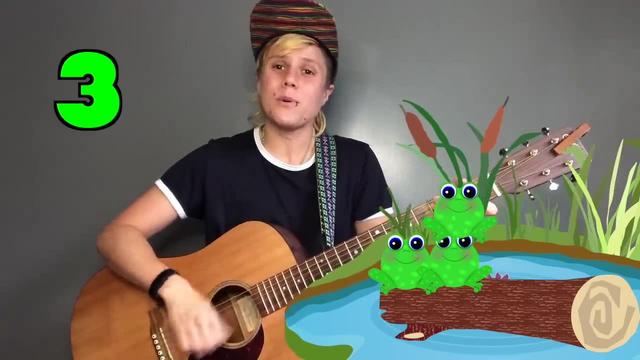 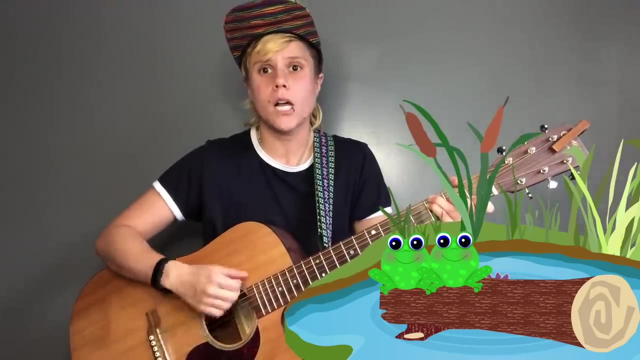 Set out a speckled log Eating some most delicious bugs. Yum yum. One jumped into the pool, where it was nice and cool. Now there are two green speckled frogs. Blah, blah, blah. Two green and speckled frogs. 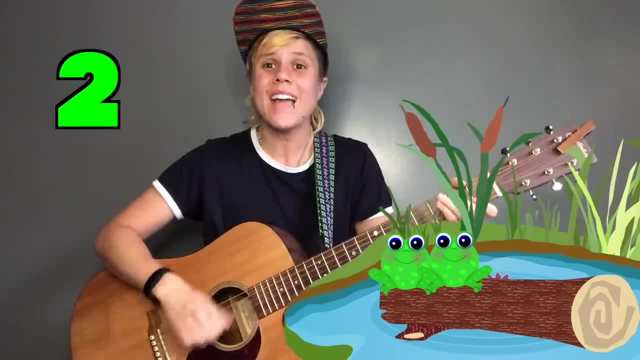 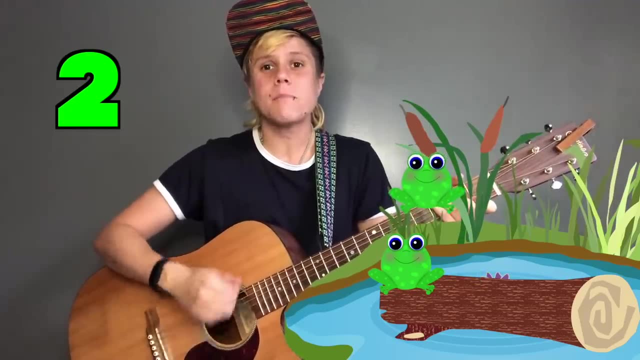 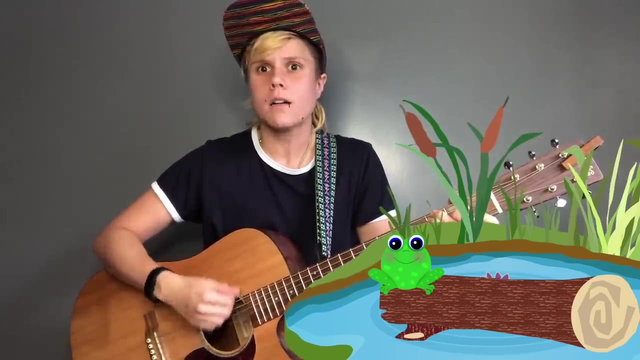 Set out a speckled log, Sat on a speckled log eating some most delicious bugs, Yum yum. One jumped into the pool, where it was nice and cool. Now there is one green speckled frog, Glub glub. 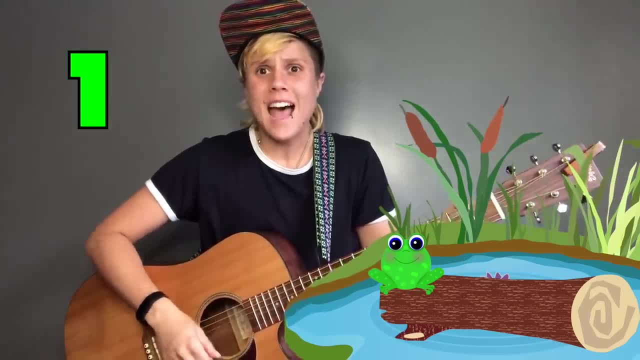 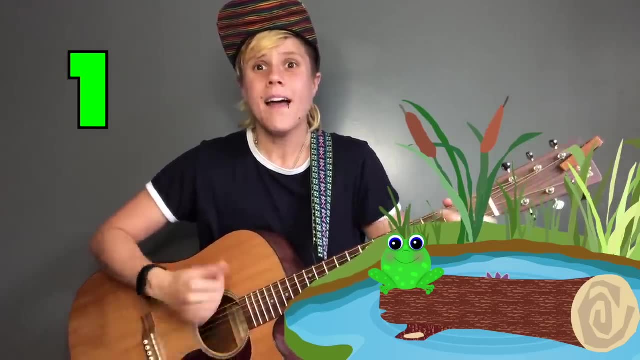 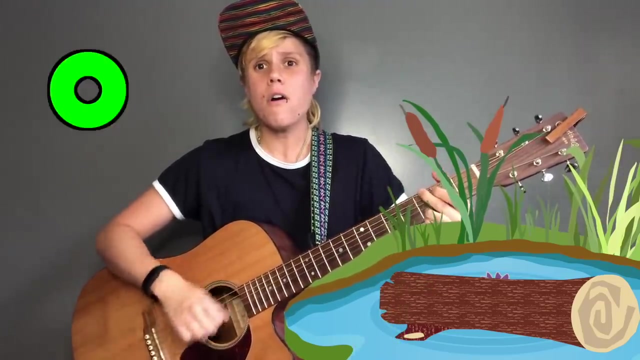 One green and speckled frog sat on a speckled log eating some most delicious bugs, Yum yum. One jumped into the pool, where it was nice and cool. Now there are no green speckled frogs. Glub, glub. 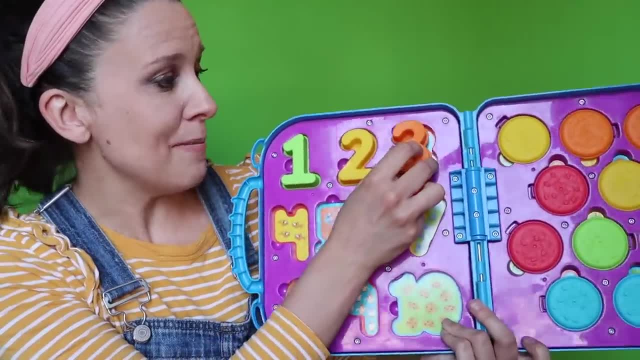 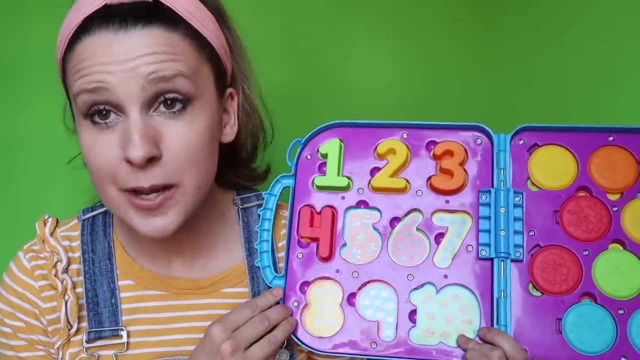 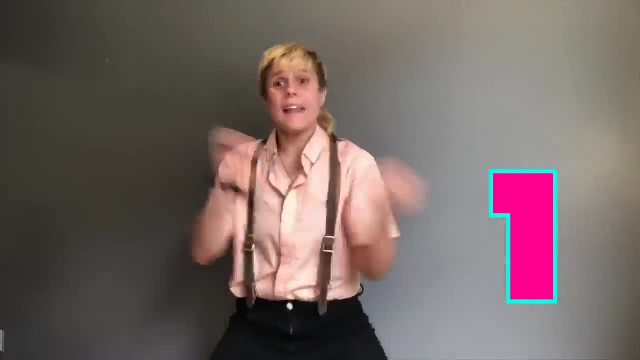 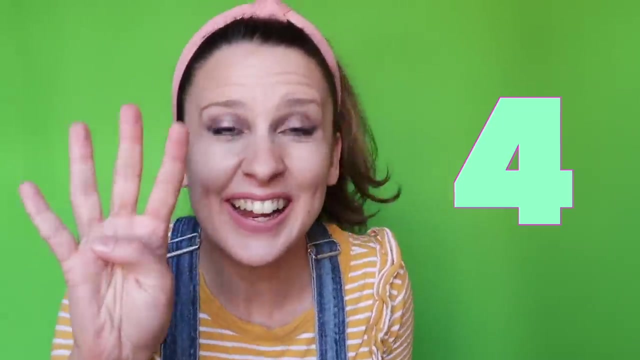 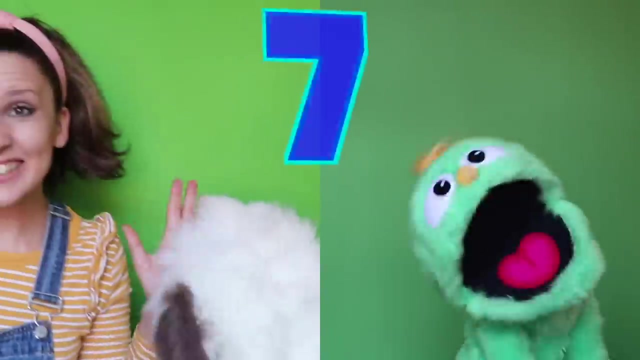 Guess what We did it? Three came back, Push, And four came back, Wow, Let's keep singing number songs so we can get more numbers for our puzzle. One, Two, Three, Four, Five, Six, Seven, Eight. 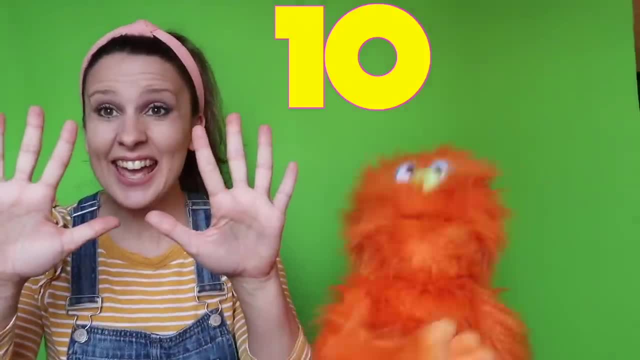 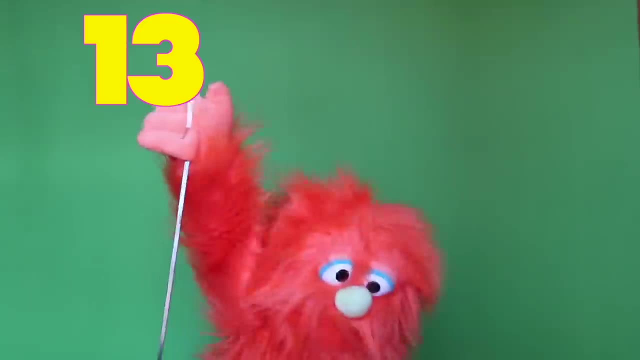 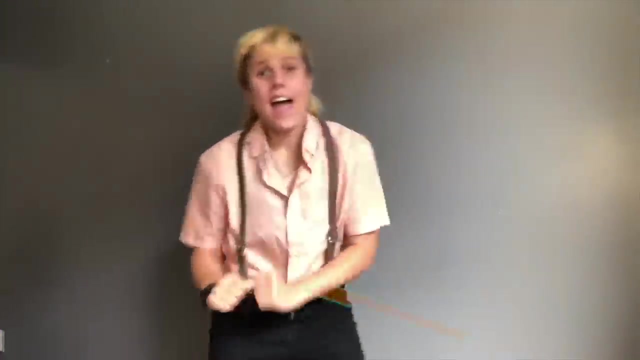 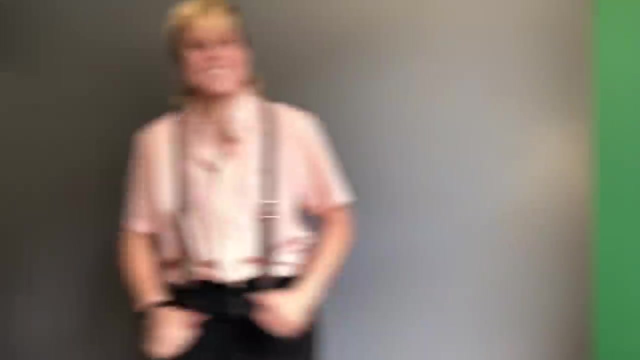 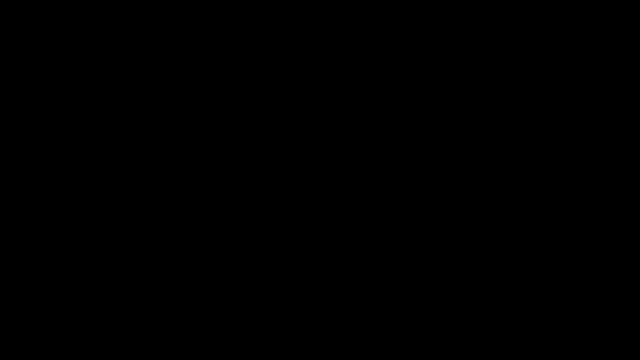 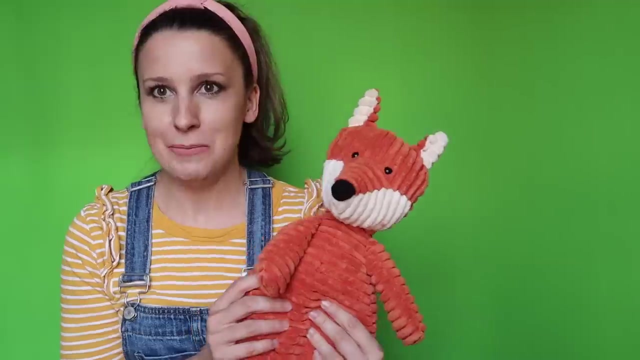 Nine, Ten, Eleven, Twelve, Thirteen, Thirteen, Fourteen, Fifteen, Sixteen, Seventeen, Eighteen, Nineteen, Twenty, Can you get out a stuffed animal? It's going to be so much fun Get out a stuffed animal, and we're going to try and balance it. 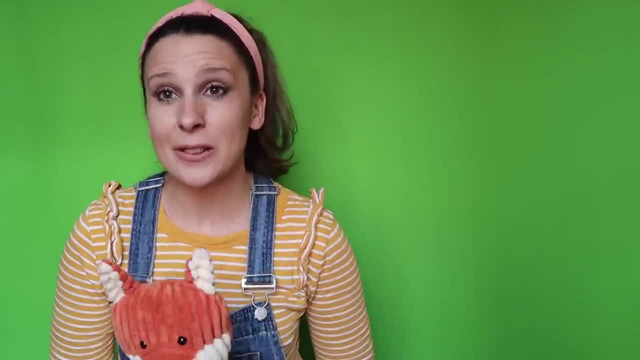 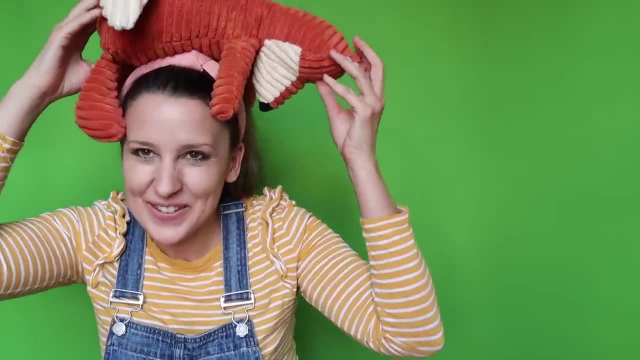 I learned this from my friend, Ms Lovenhofer, And this is how you do it, And this song is by Lori Berkner, a wonderful children's songwriter that we love. Can you put your stuffed animal on your head, So silly? Can you balance it? 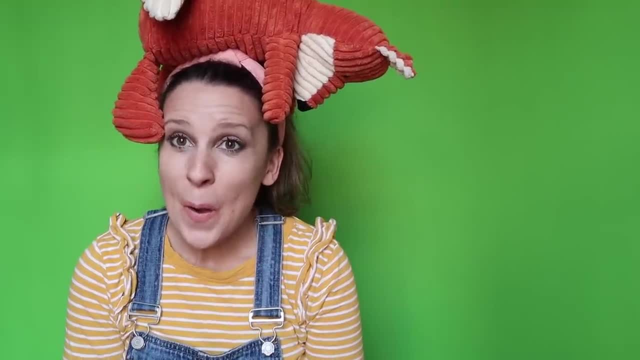 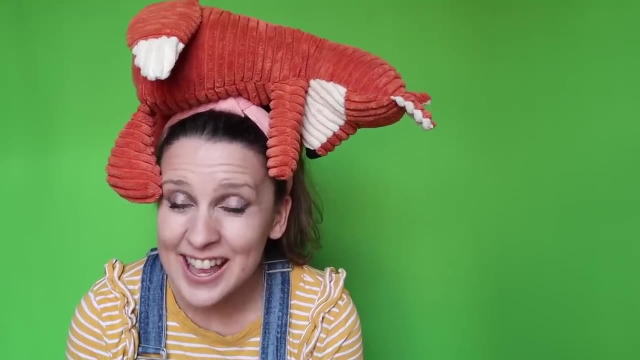 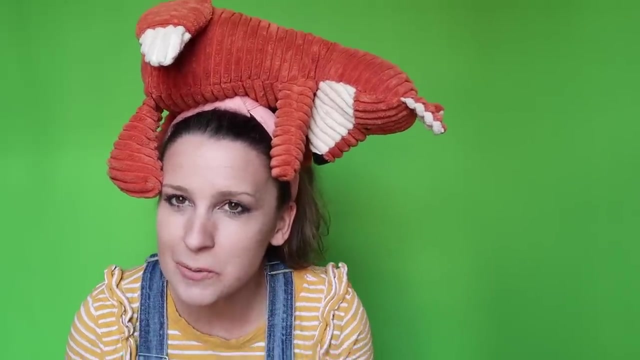 And now let's sing. Rachel's got a fox on her head. Rachel's got a fox on her head. Rachel's got a fox on her head. She keeps it there all day. Wow, I wonder if we could balance it another place. How about my shoulder? Can you try your shoulder? 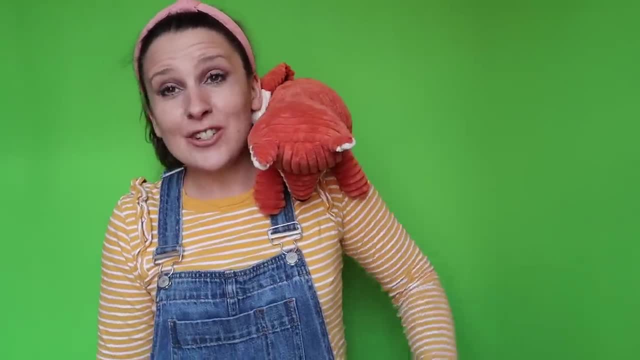 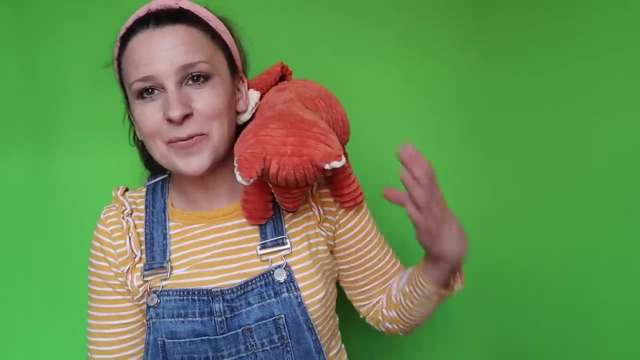 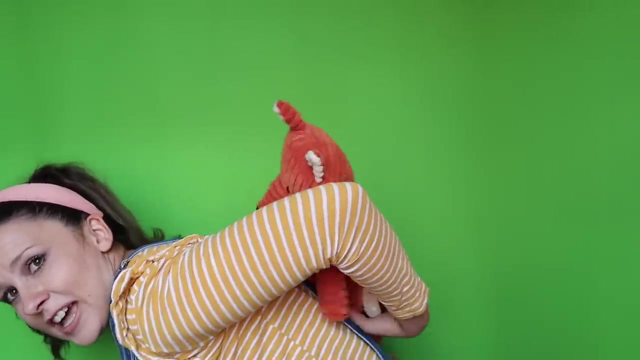 Rachel's got a fox on her shoulder. Rachel's got a fox on her shoulder. Rachel's got a fox on her shoulder. She keeps it there all day. Wow, Let's try our backs. Could you do that? Oh, it's pretty hard. I'm going to try, Always. keep trying. 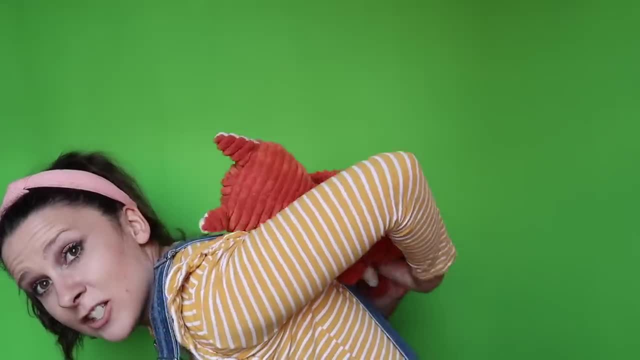 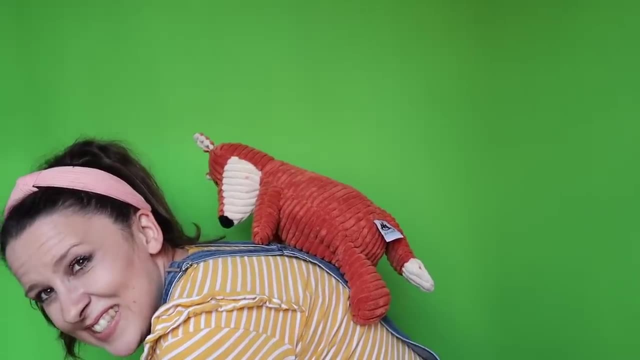 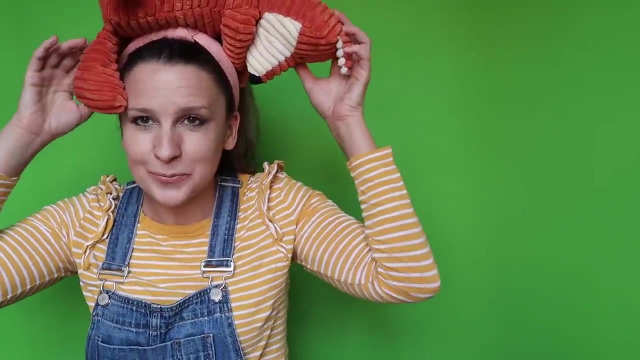 Yay, Rachel's got a fox on her back. Rachel's got a fox on her back. Rachel's got a fox on her back. She keeps it there all day. That's so fun. Let's have you put your stuffed animal on your head and then we'll sing about you. 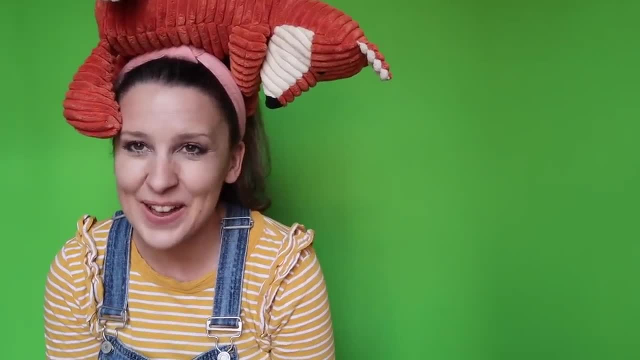 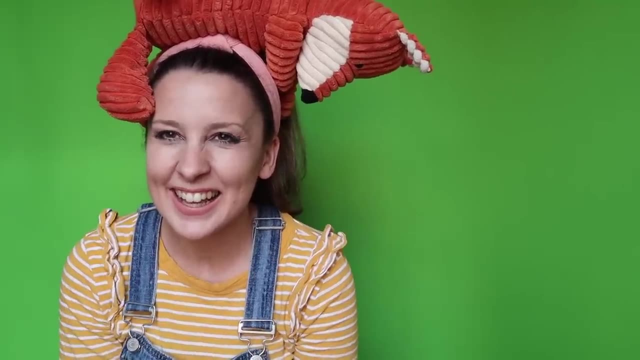 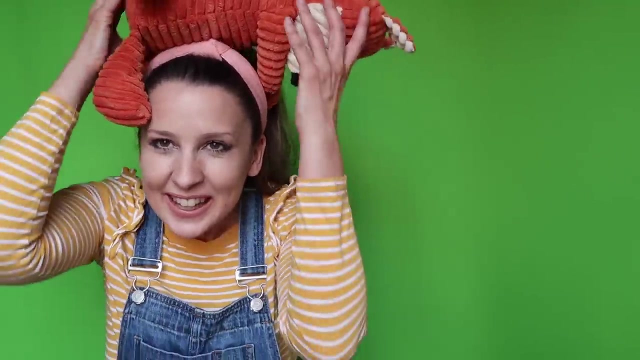 And you can fill it in Ready and go. Got a on their head. Got a on their head. Got a on their head. They keep it there all day. I was singing about you and your animal. Yeah, that's so fun. Let's try one more time on our head. 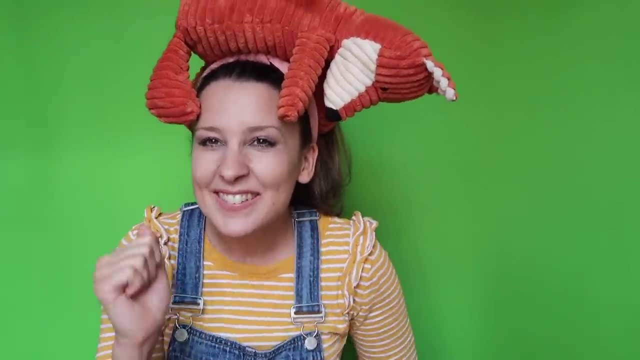 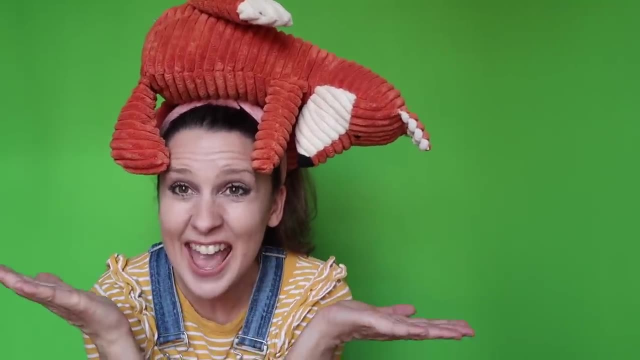 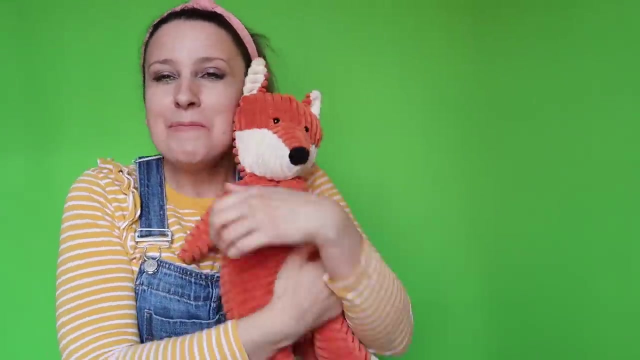 Rachel's got a fox on her head. Rachel's got a fox on her head. Rachel's got a fox on her head. She keeps it there all day. Wow, That was so fun. Let's give our stuffed animal a big hug and a kiss. 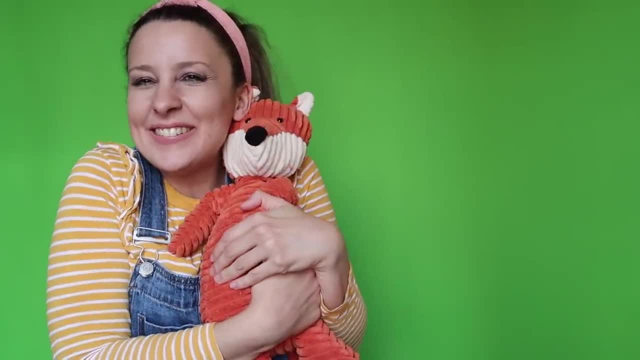 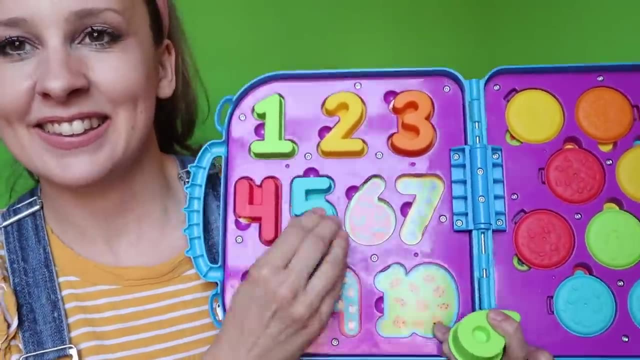 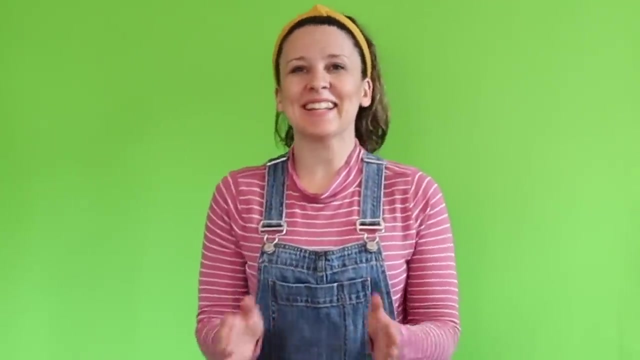 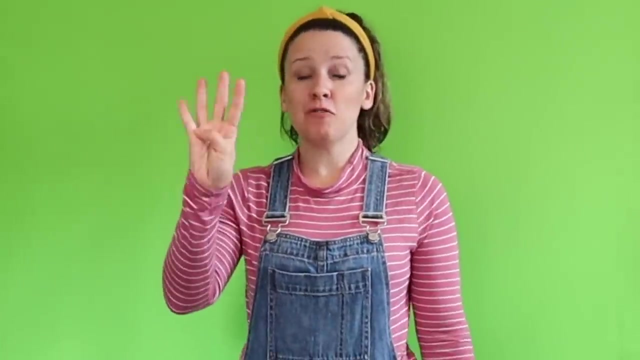 I love you. Hooray, Guess who came back. Number five and number six. We're almost there. Let's get a steady beat going. One, two, buckle my shoe. Three, four, shut the door. Five, six: pick up sticks. 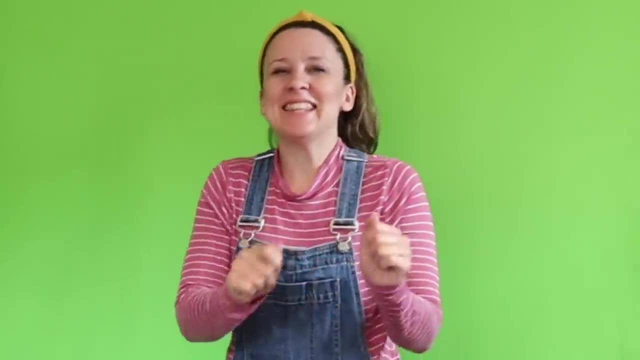 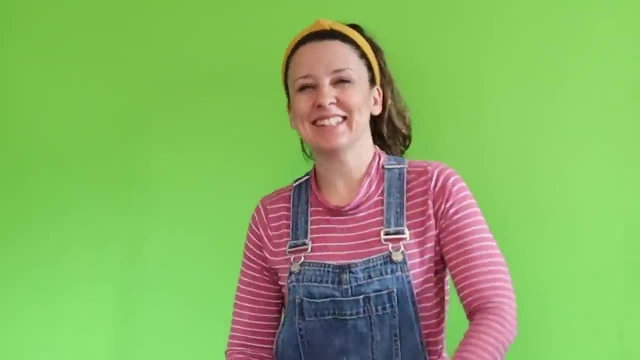 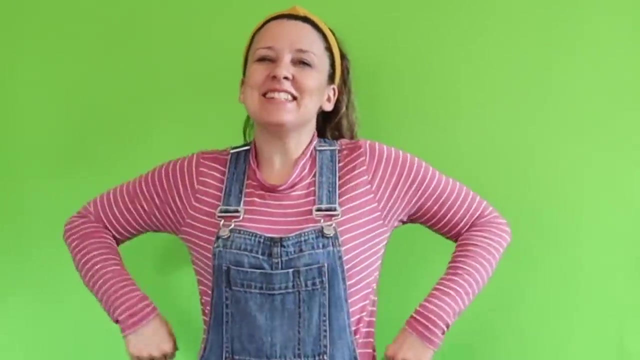 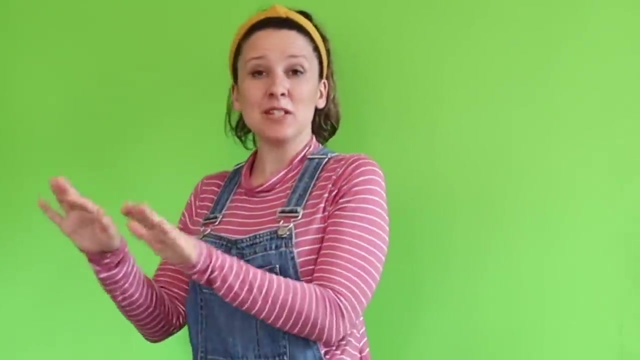 Seven, eight, lay them straight. Nine, ten, do it again. Yay, Let's do it again. One, two, buckle my shoe. Three, four: shut the door. Five, six, pick up sticks. Seven, eight, lay them straight. 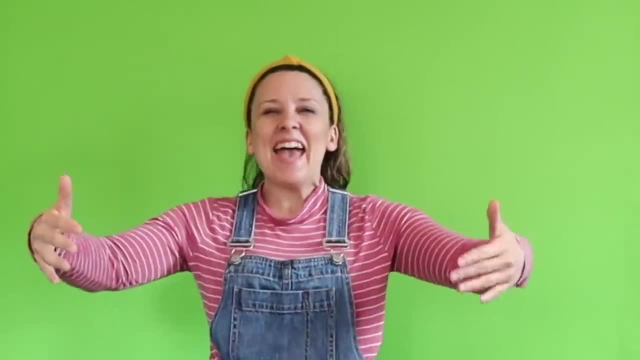 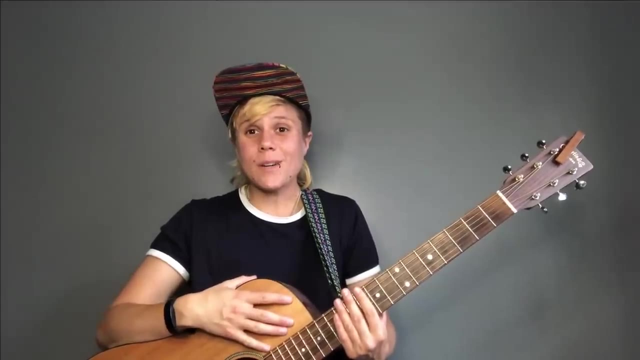 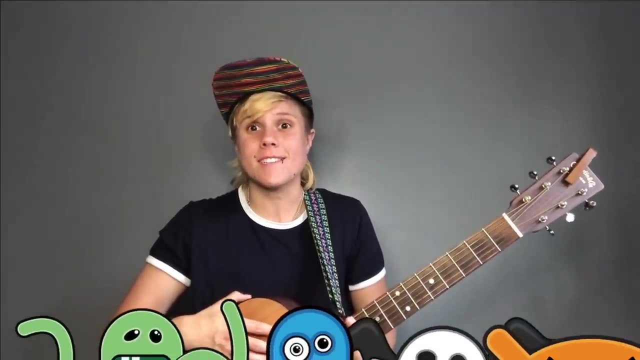 Nine, ten, a big red. hey, Red hands, Great job, Hey everyone. The next song we're going to do is by Feist. She went on Sesame Street and wrote a song about counting monsters, So we're going to play it right now. 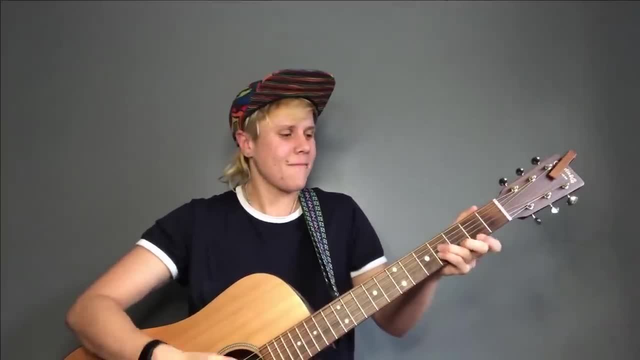 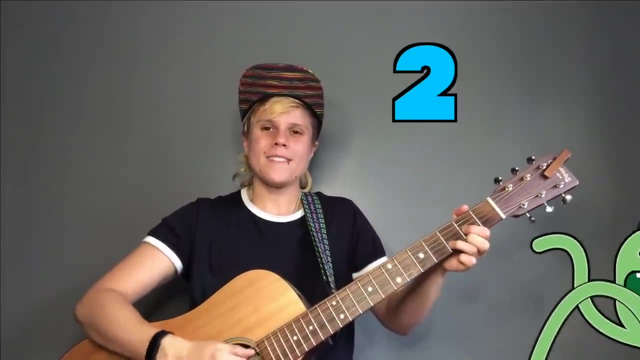 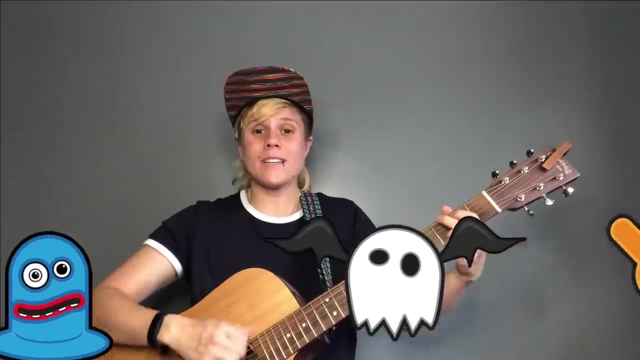 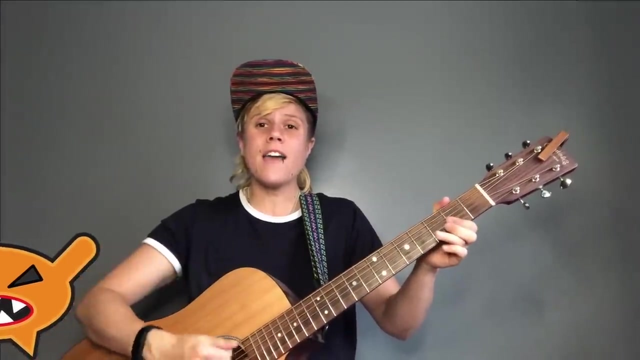 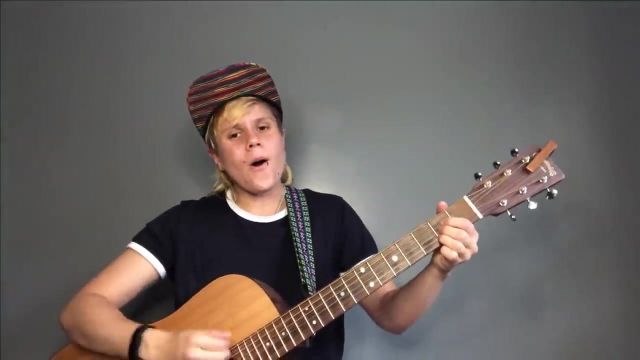 One, two, three, four monsters walking across the floor. I love counting, counting to the number four. Oh, you're counting. you're counting with me To one less than five and one more than three. Oh, oh, oh, we're counting to four. 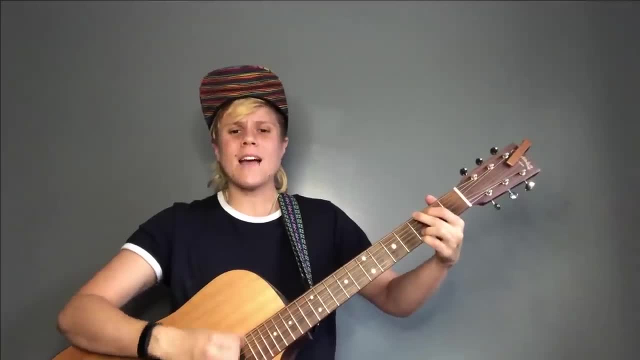 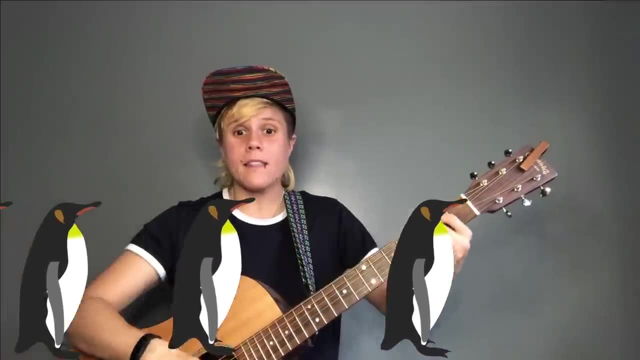 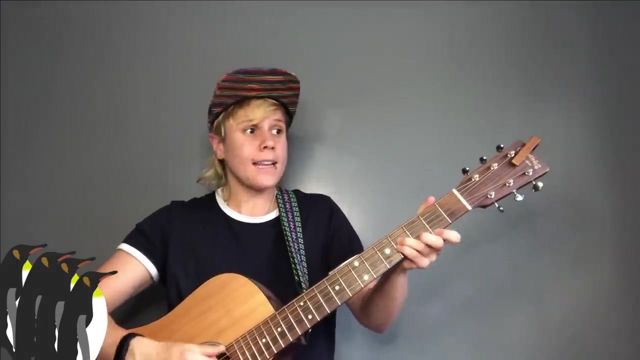 Oh, oh, oh. let's count some more. One, two, three, four penguins that went by the door. I love counting, counting to the number four. I see four here and I see four there, My favorite number: nothing can compare. 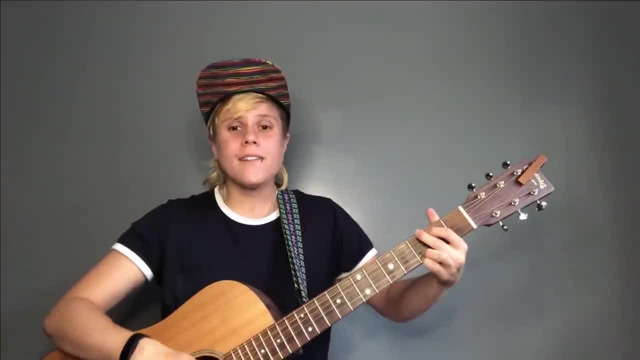 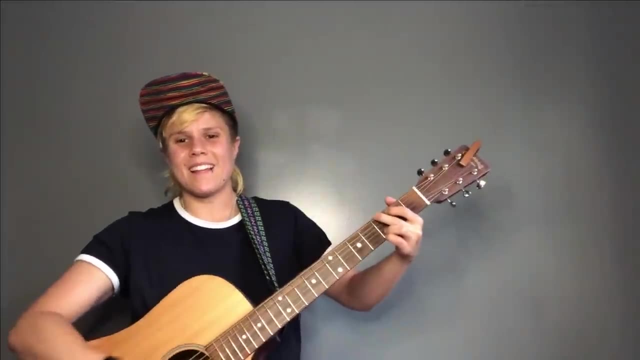 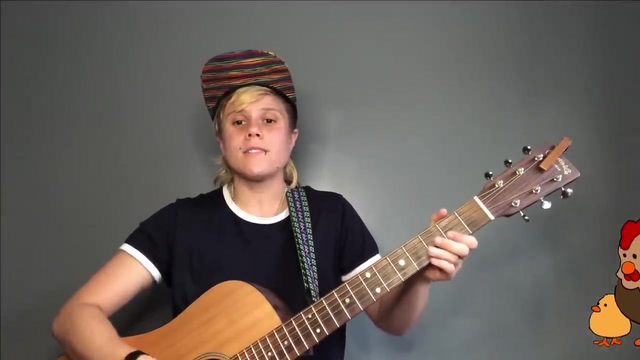 Oh oh oh, we're counting to four. Oh oh oh, let's count some more. One, two, three, four chickens back from the shore. I love counting, counting to the number four. Oh oh, oh, we're counting to four. 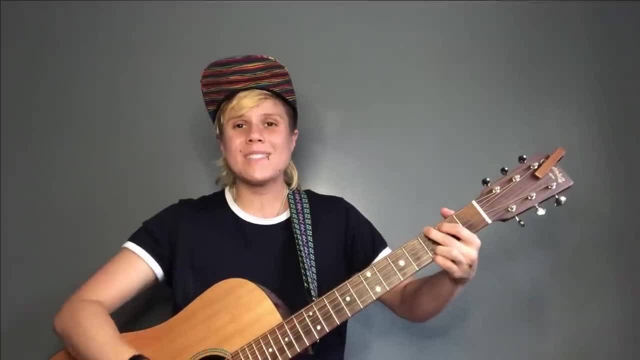 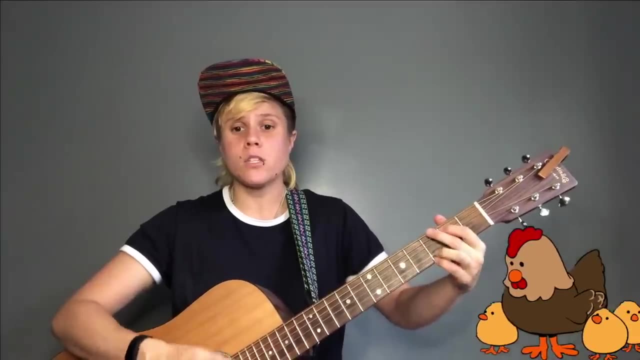 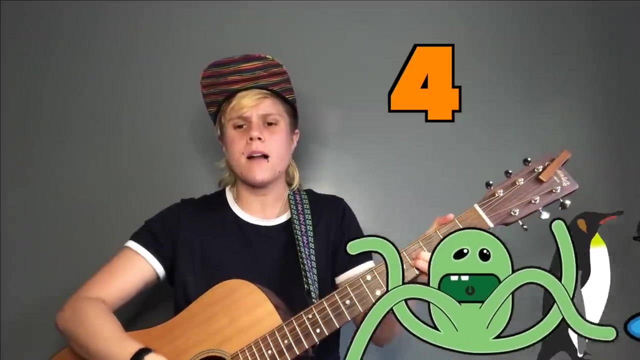 Oh, oh oh, let's count some more. One, two, three, four chickens back from the shore. One, two, three, four penguins that went by the door. One, two, three, four monsters walking across the floor. 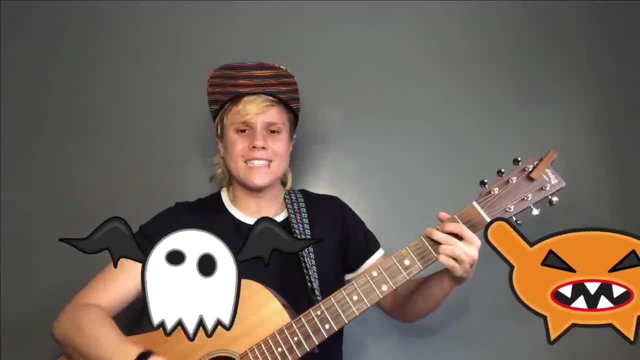 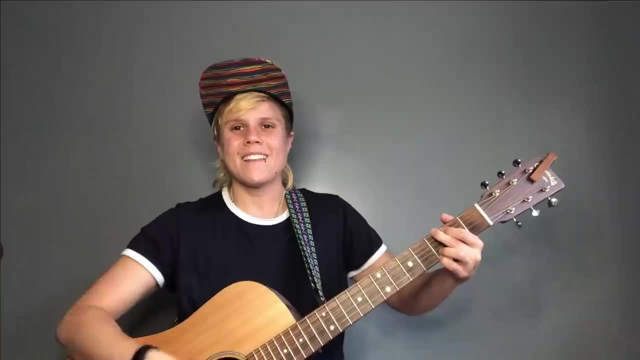 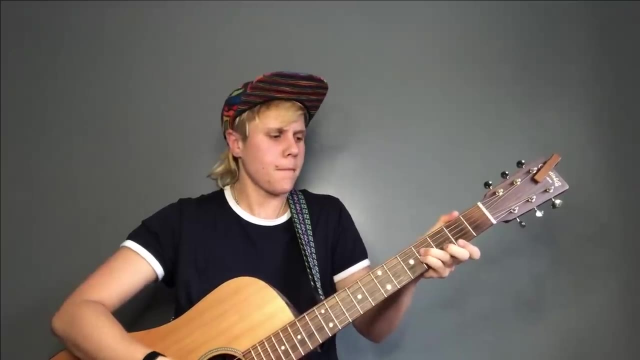 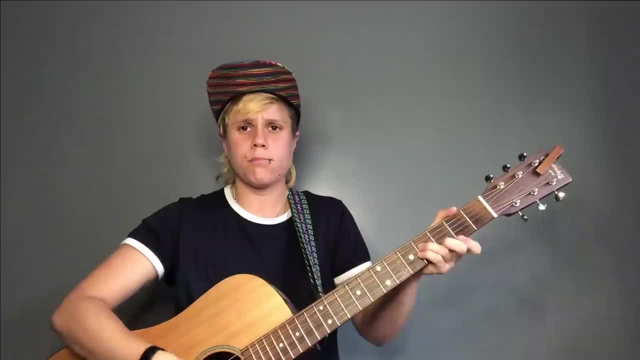 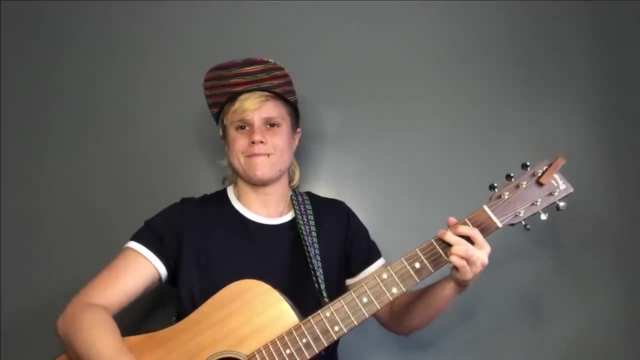 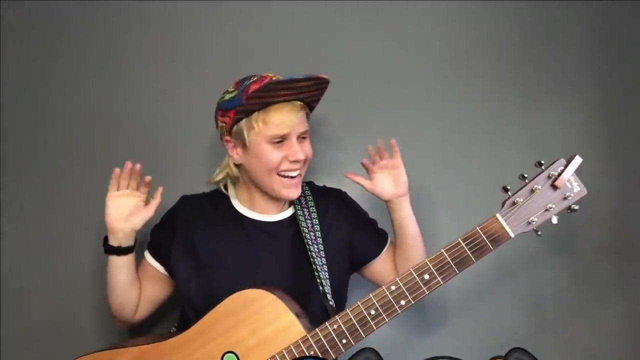 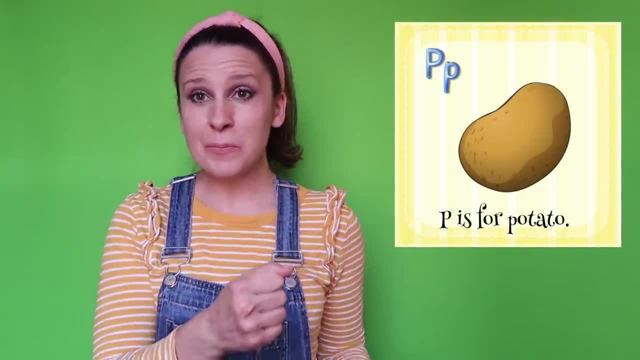 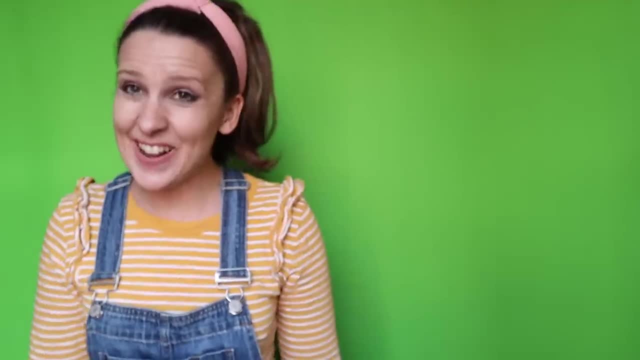 Let's pretend our hands are potatoes. One potato, two potato, three potato four, Five potatoes, six potatoes, Seven potato more. Good job, Let's try it with a friend. One potato, two potato, three potato, four. 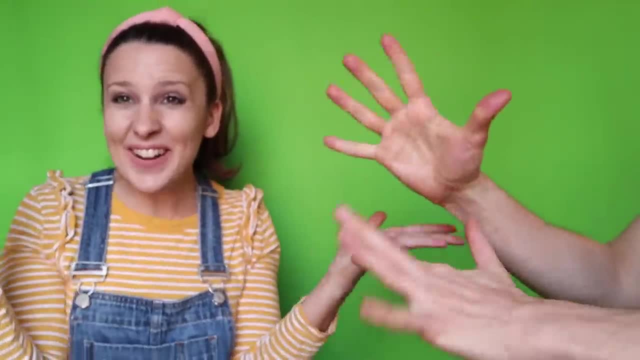 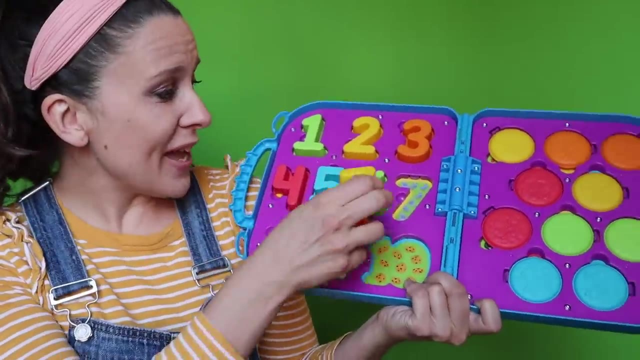 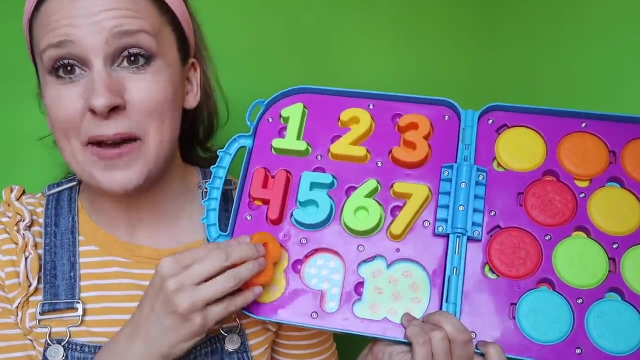 Five potatoes, six potatoes, seven potato more. Whoa, That was so fun. Good job counting potatoes. Yay, Guess who came back. Seven came back, Eight came back- Push it in- And number nine came back. Wow, 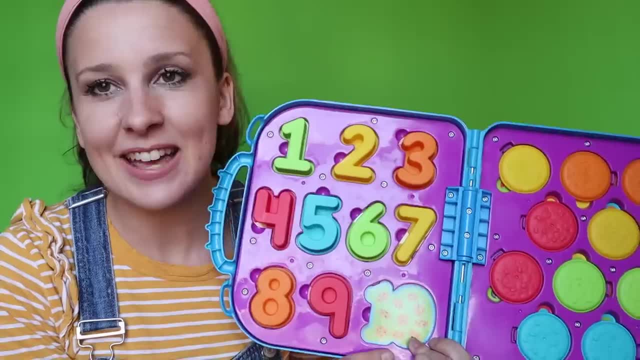 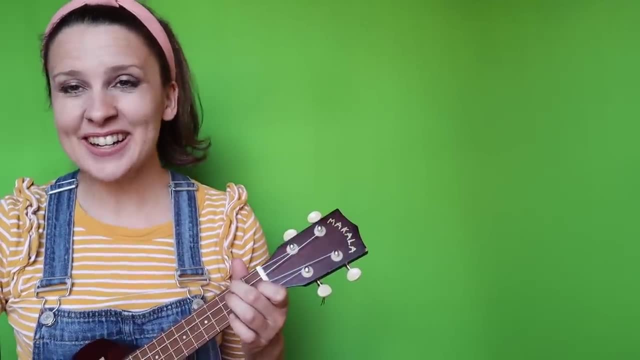 We only have one more number. Let's sing another really great number song and I know number ten will come back. Hey, everyone Guess what? it's time for Word of the day. Yay, The word of the day. Hi, Herbie. 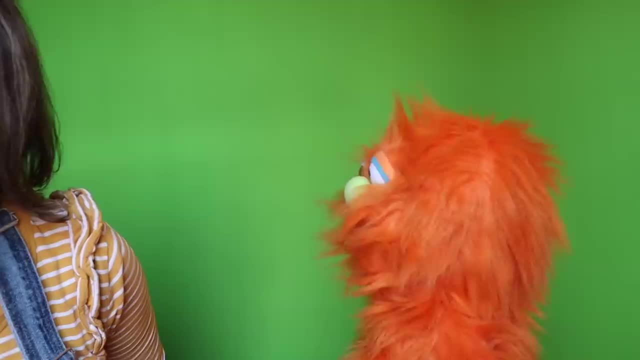 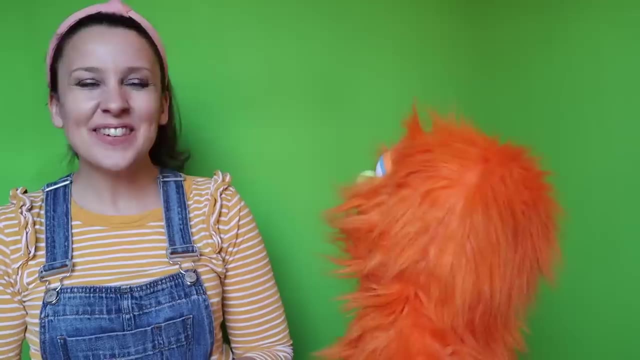 This is my favorite part. I love this part too. Me too. The word of the day is beat. Oh delicious, Herbie. Yeah, I love roasted beets. Not that kind of beet. Beet salad, No, a musical beet. 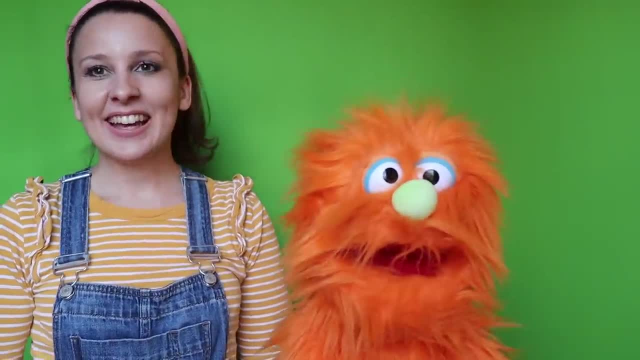 Beet soup. It's not a kind of beet you can eat. Oh, okay, It's a musical beet. Oh, The musical beet is the steady pulse in the music. Is that a beet you can eat? Do you like that rhyme? I do. 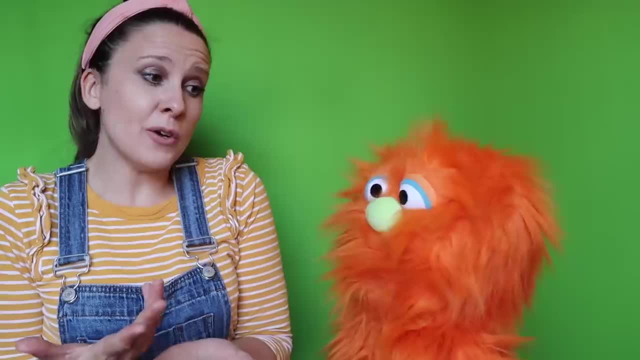 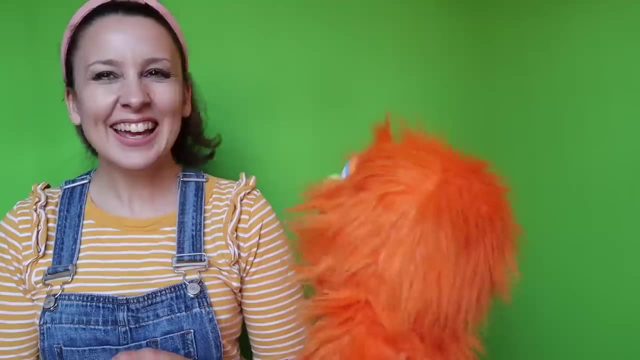 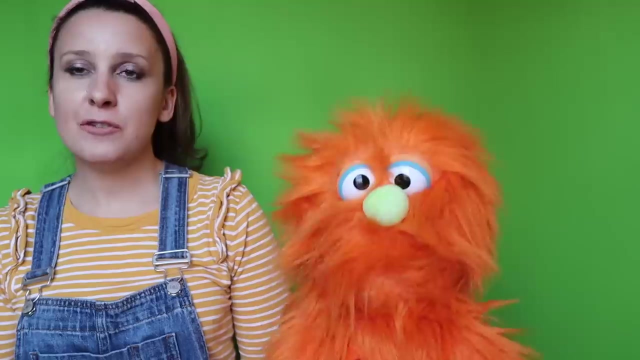 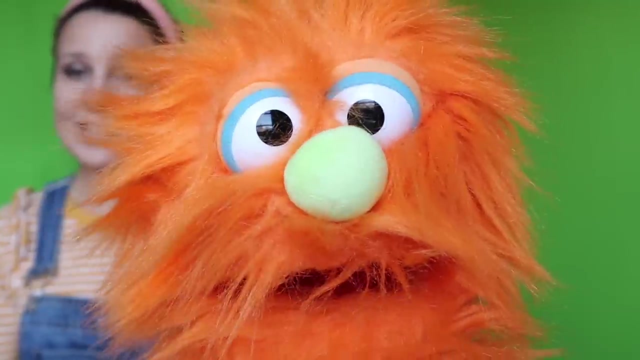 Thanks. So what in your body has a steady beat? A steady beat, One, Two, Three, Four, Five, Six, Seven, Eight, Nine, Ten, Eleven, Twenty, a steady beat. Part of our body has a steady beat. Do you know? I don't know. What do you think it is? 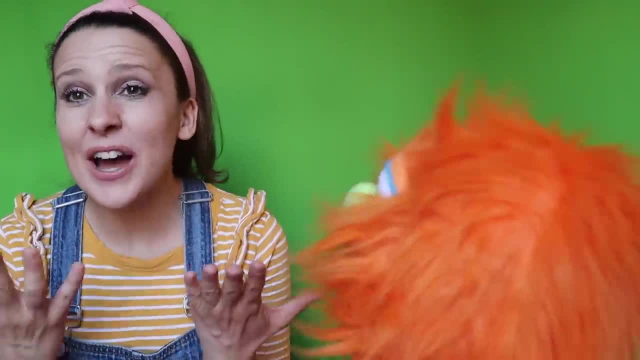 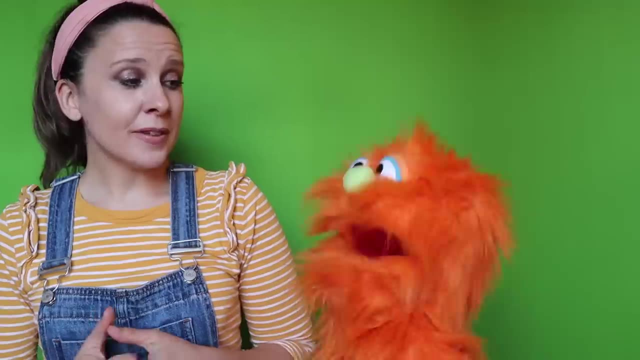 Oh, the heart. Yes, you guys are right, It's the heart. It has a steady beat. Yeah, And music has a steady beat, like your heart, Like the heart. Let's sing a song and you'll march to the beat. 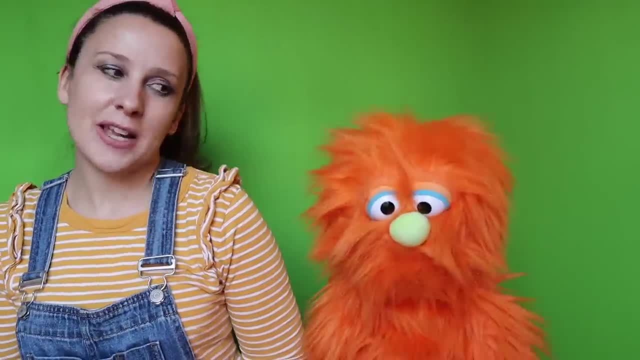 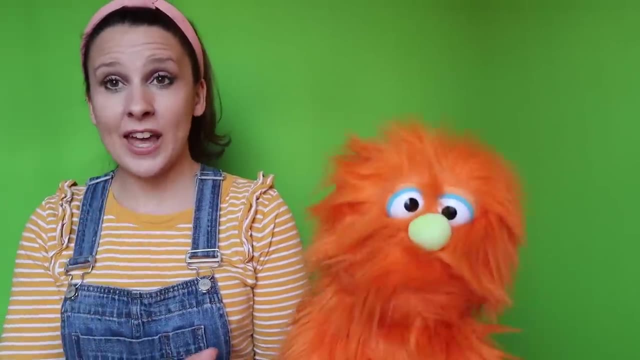 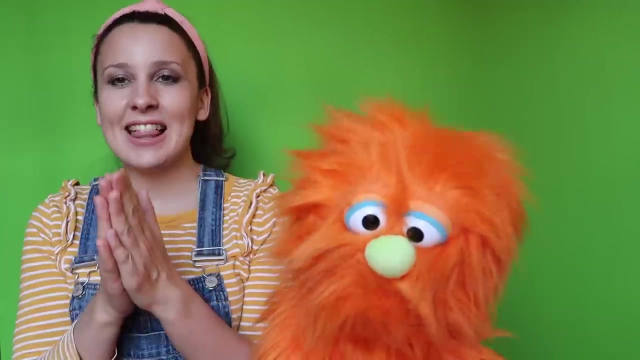 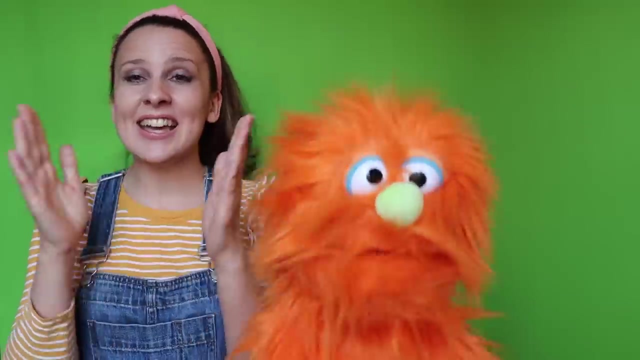 and I'll clap: Okay. Okay, All right, Let's do our ABCs. Do you know your ABCs? Great, Me too. One, two ready. go A, B, C, D, E, F, G, H, I, J, K, L, M, N, O, P, Q, R, S, T, U, V, W, X, Y and Z. 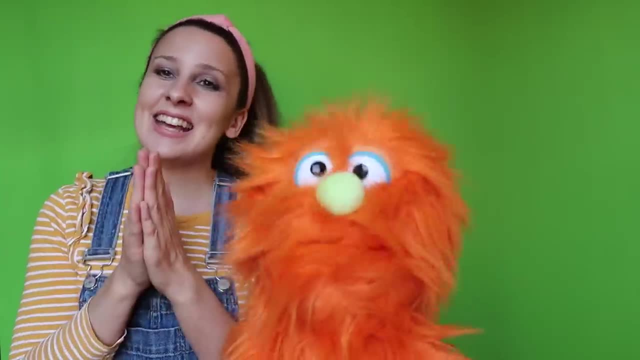 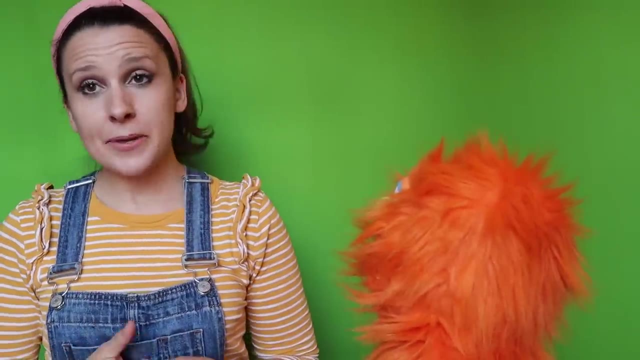 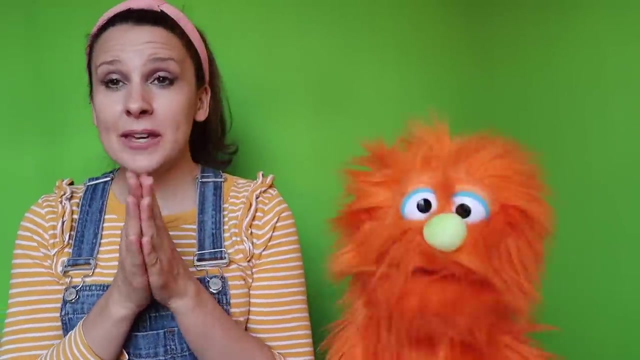 Now, I know my ABCs. Next time won't, Don't you sing with me? Yay, Now let me ask you something. Yeah, Did that beat change or stay the same? It stayed the same. Yeah, it stayed the same. Yeah, I got it right. The beat has a steady pulse. 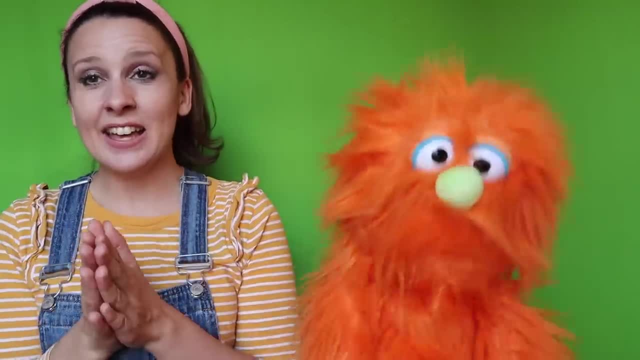 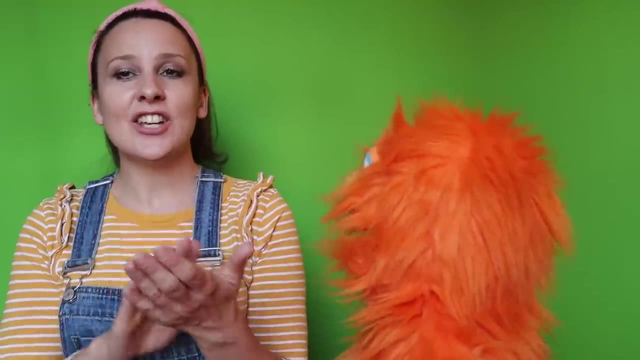 that stays the same. That stays the same. Yeah, The rhythm does change. Listen to this: A, B, C, D, E, F, G, H, I, J, K, L, M, N, O, P, Q, R, S, T, U, V. 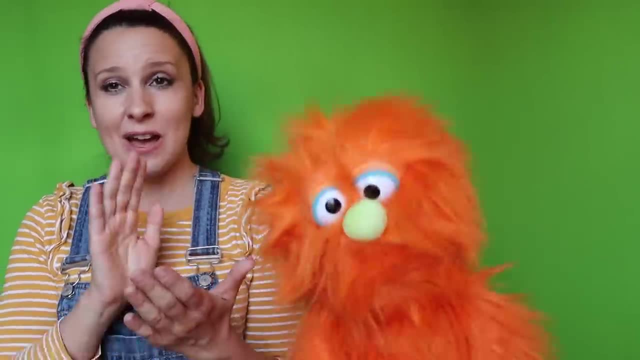 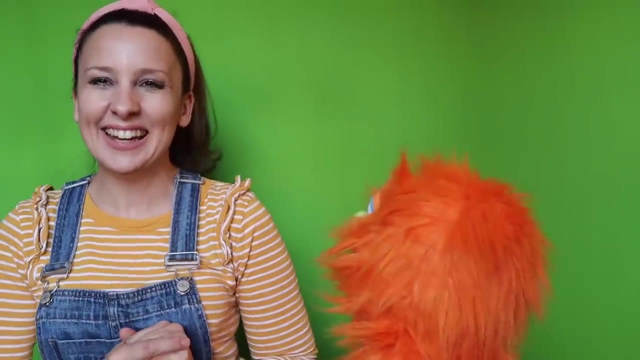 W, X, Y and Z. Now I know my ABCs. Next time won't you sing with me L M N O, L M N O. Yeah, it goes really fast. The next song we're going to sing is about a tiny little. 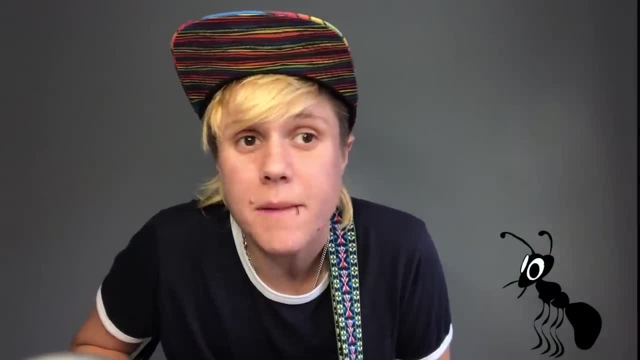 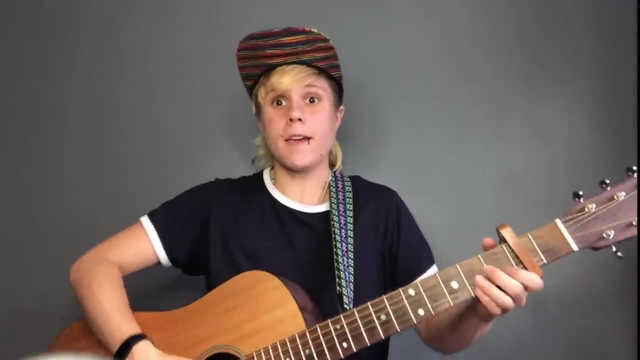 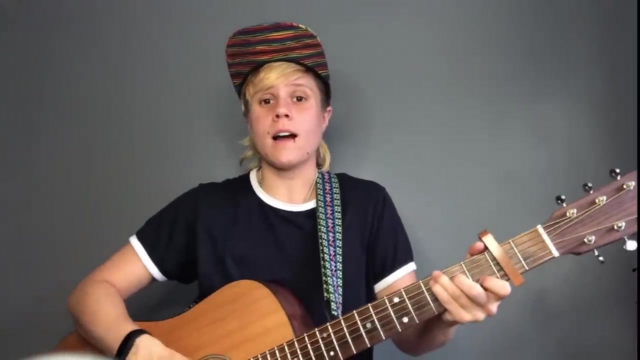 bug called an ant. We're going to sing a song about them marching and we're going to count them as they march. Can you march with me? Let's go? Here we go. The ants go marching one by one, Hurrah, hurrah. The ants go marching one by one, Hurrah, hurrah. 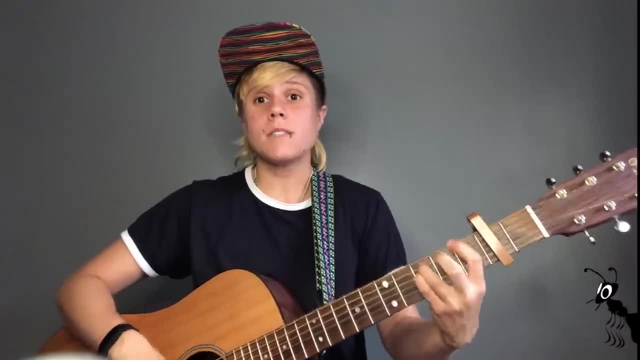 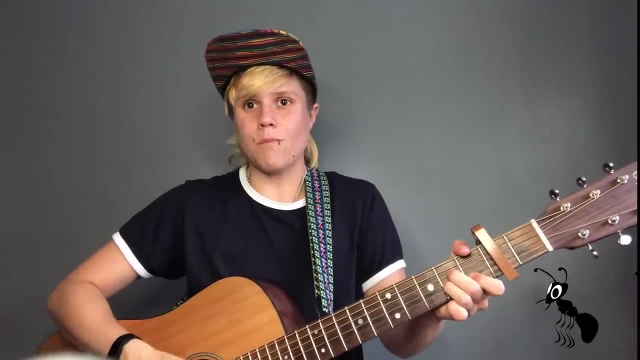 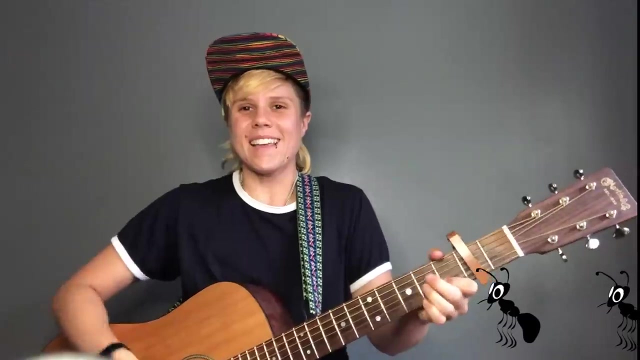 The ants go marching one by one. The little one stopped his thumb and they all go marching down to the ground to get out of the rain. Boom, boom, boom, boom, boom, boom, boom. The ants go marching two by two. Hurrah, hurrah. The ants go marching two by two. 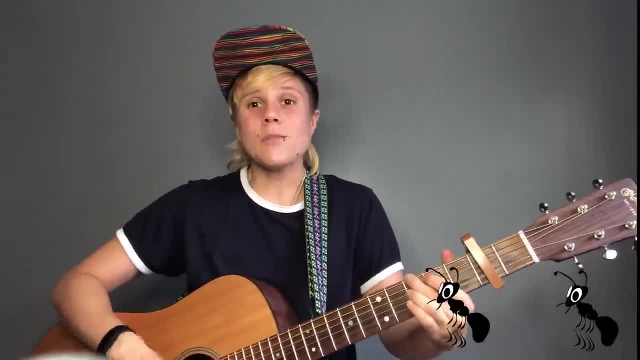 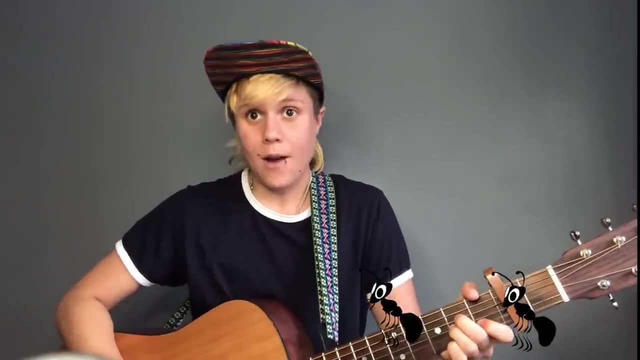 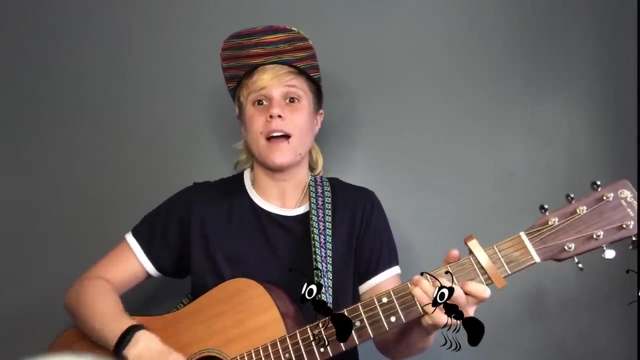 The little one stopped to tie his shoe and they all go marching down to the ground to get out of the rain. Boom, boom, boom, boom, boom, boom, boom. The ants go marching three by three. Hurrah, hurrah, The ants go marching three by three. Hurrah, hurrah, The ants go. 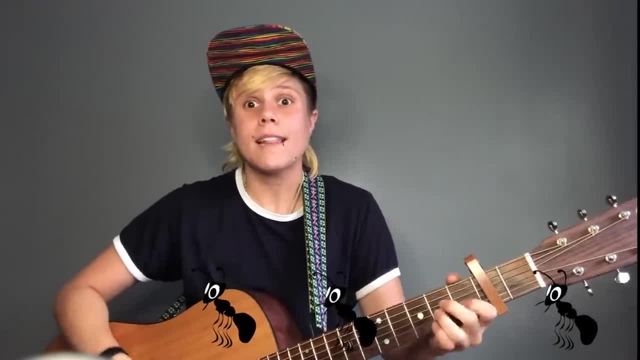 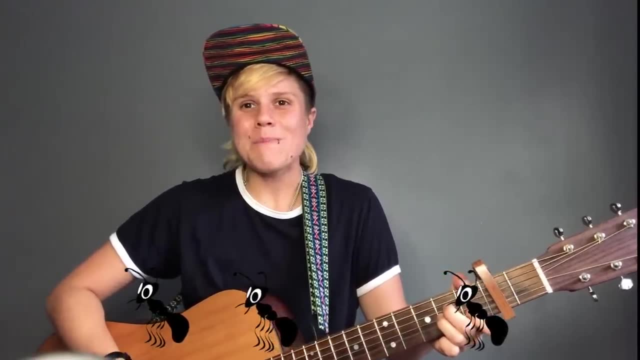 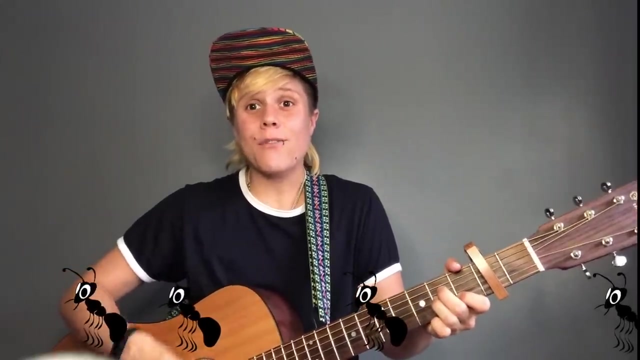 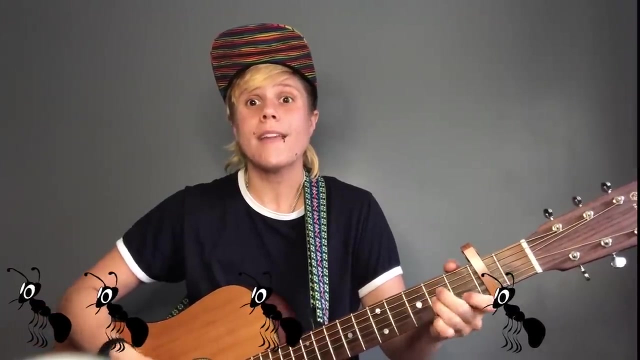 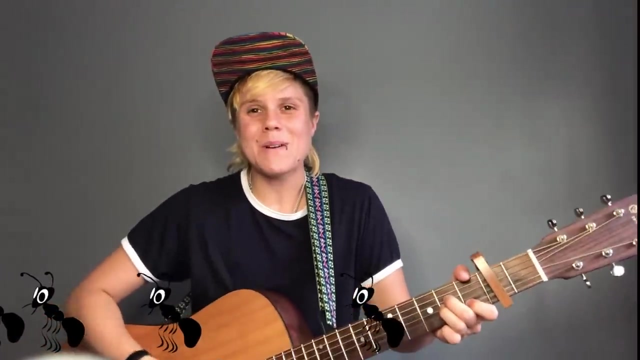 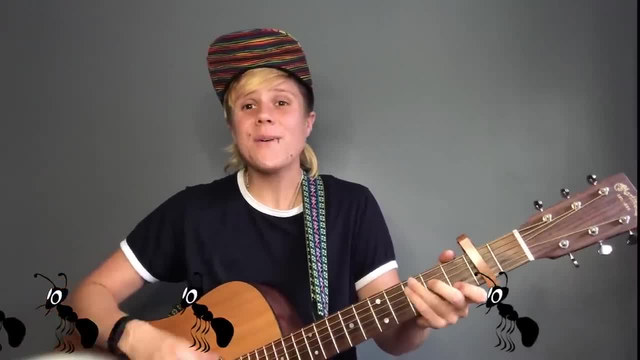 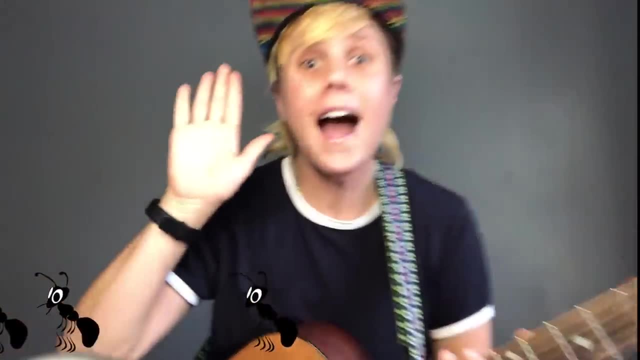 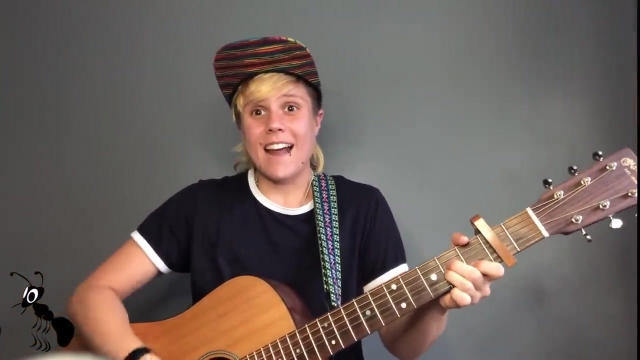 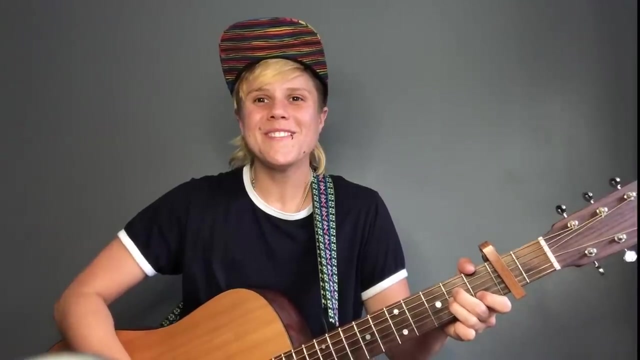 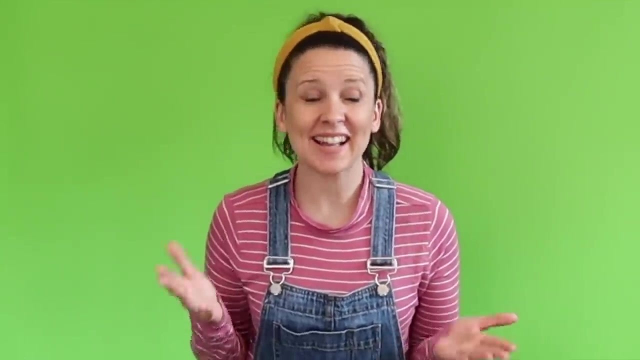 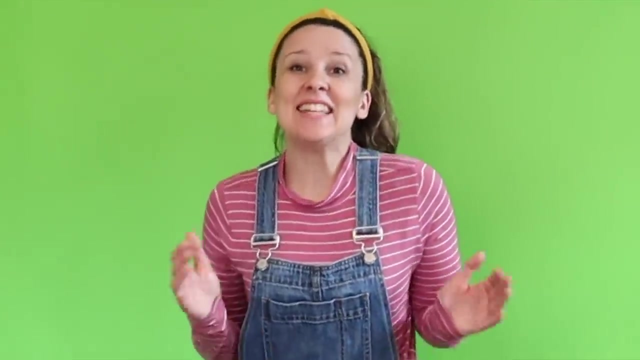 Y'all did so good. Do you have a teddy bear? Wow, If you want, you can get out your teddy bear for this rhyme: Teddy bear, teddy bear, turn around. Teddy bear, teddy bear, touch the ground. 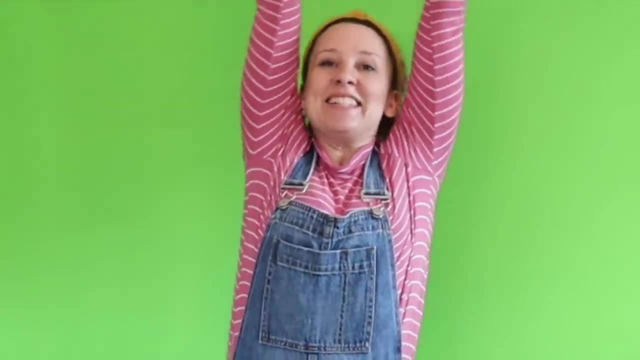 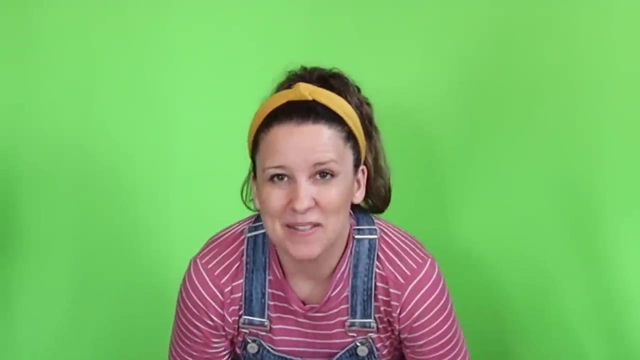 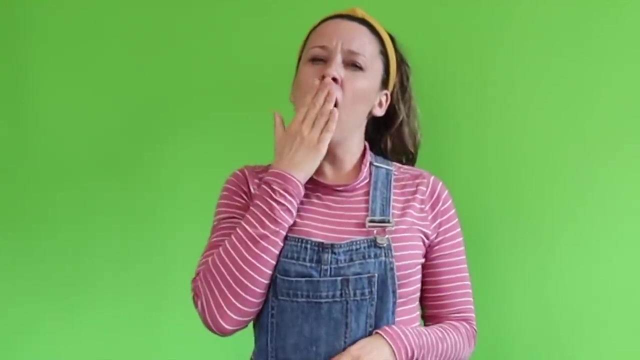 Teddy bear teddy bear. reach up high. Teddy bear, teddy bear, touch the sky. Teddy bear, teddy bear. bend down low. Teddy bear teddy bear, touch your toes. Teddy bear teddy bear. go to bed. Teddy bear teddy bear, rest your head. 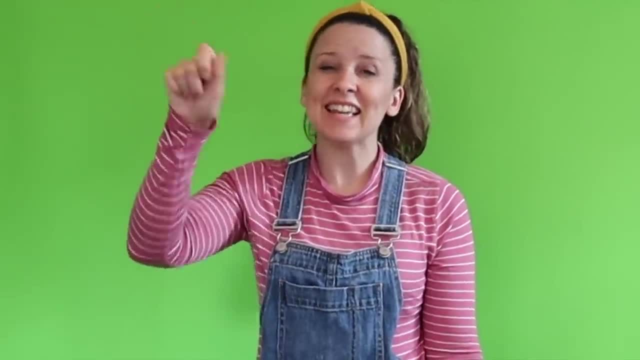 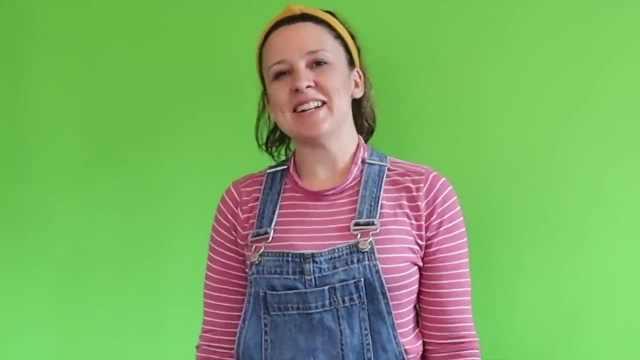 Teddy bear. teddy bear turn off the light. Click Teddy bear. teddy bear say good night. Oh, the teddy bear's so tired. Pretend to go to sleep or put your teddy bear to bed. Ding, ding, ding, ding, ding. 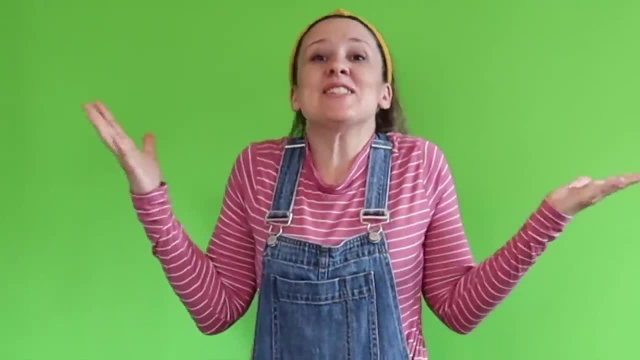 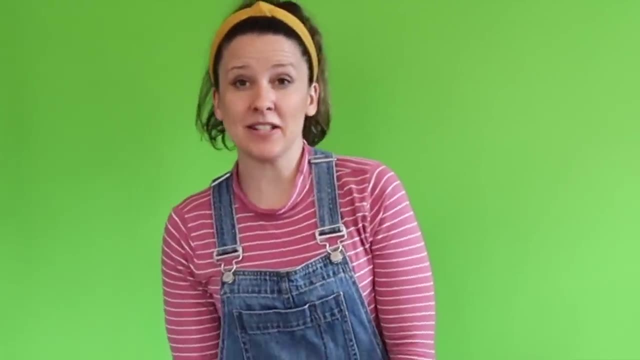 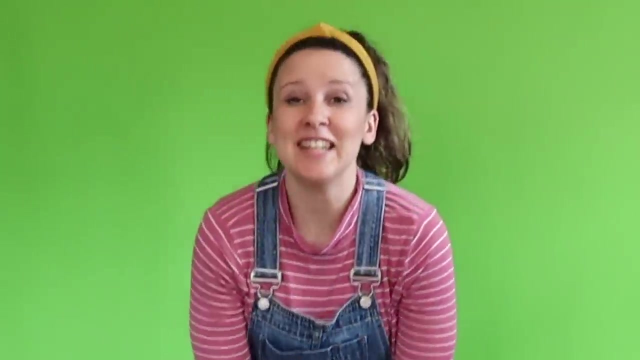 That's our alarm clock. We have to get up and sing more songs. Teddy bear, teddy bear, find your nose. Boink. Teddy bear, teddy bear, touch your toes, Oh, touch your toes. Teddy bear, teddy bear, touch your knees. Are you touching your knees? 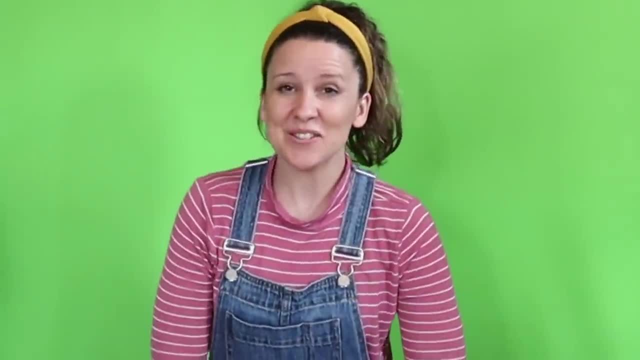 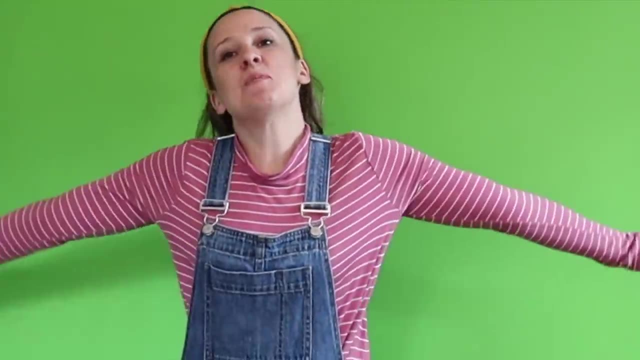 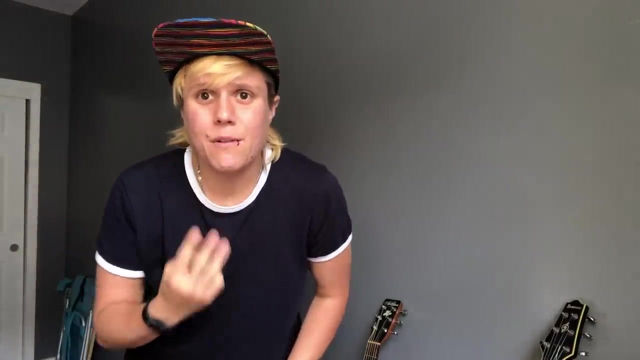 Teddy bear. teddy bear, sit down. please Are you sitting down? Good job, You're doing such a great job in music today and I'm so proud of you. Hey guys, I need your help. I thought I had three guitars, but I can't remember how to count them. 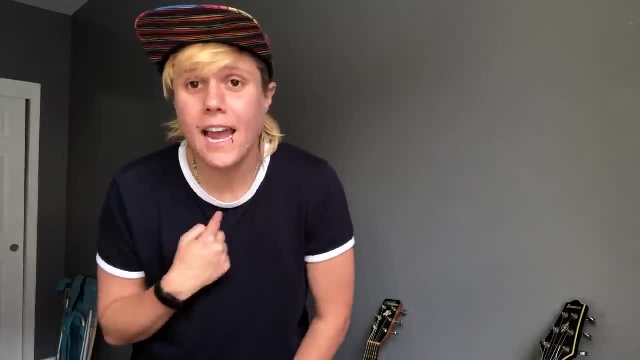 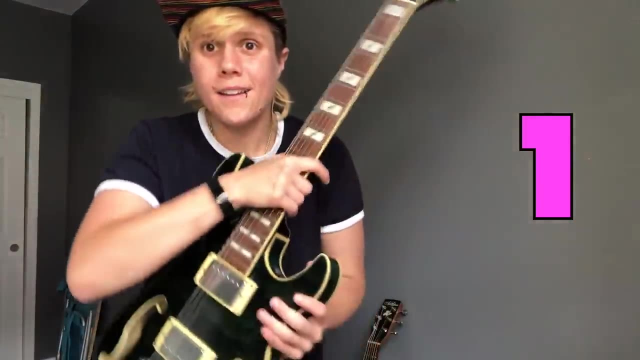 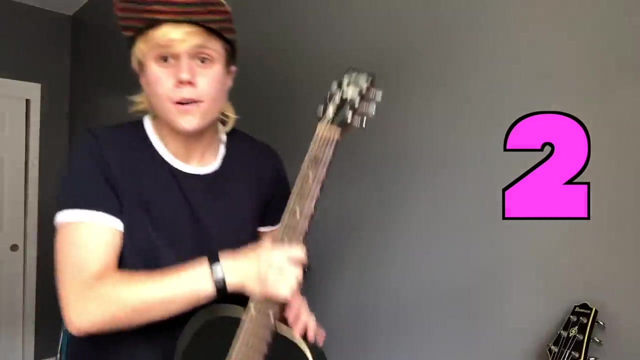 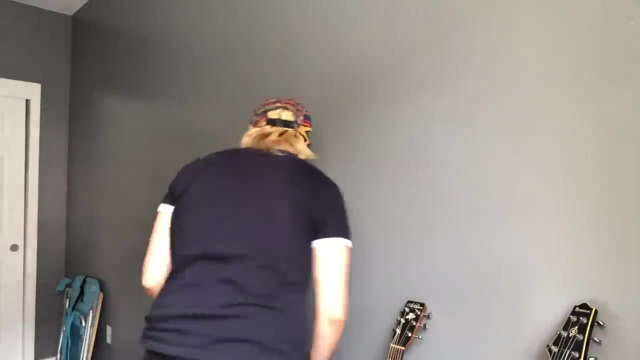 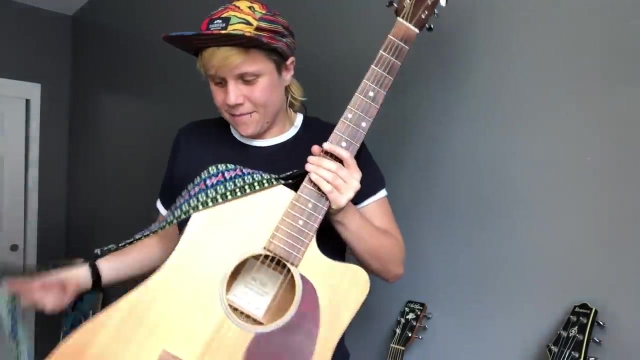 Can you help me count to three and make sure that I have three guitars? Thank you, Okay, here's one, This is an electric guitar, Here's two, This is a small acoustic guitar, and here's three. That means I have three guitars. All right, let's sing a song about my three. 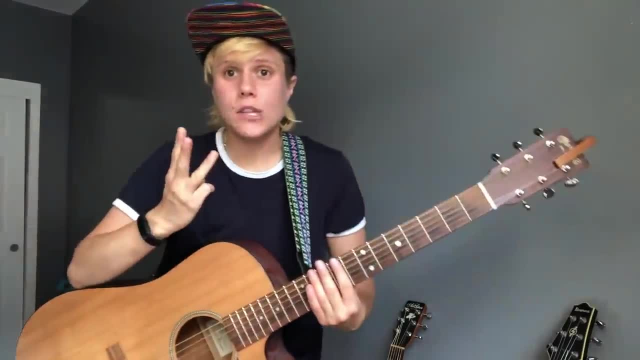 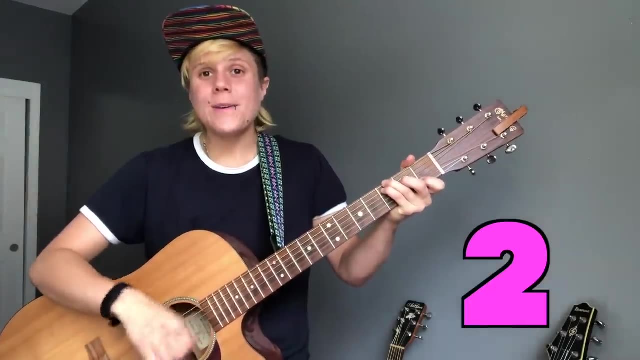 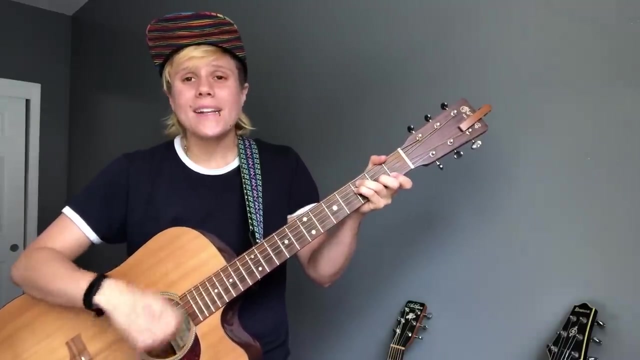 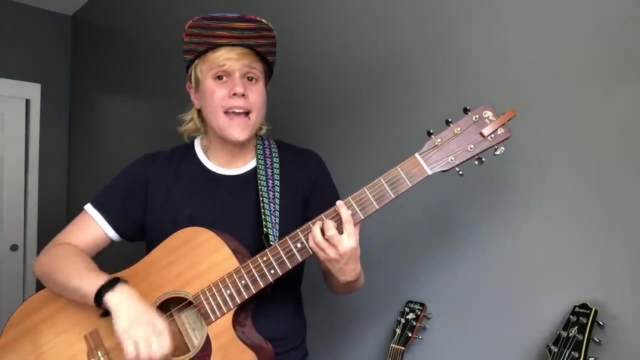 guitars. Are y'all ready? We're going to count to three and I want you to dance if you feel like it. One, two, three. One two, three rocking guitars. One, two, three rocking guitars. Play it all day, play all night. rock my way to a lullaby. 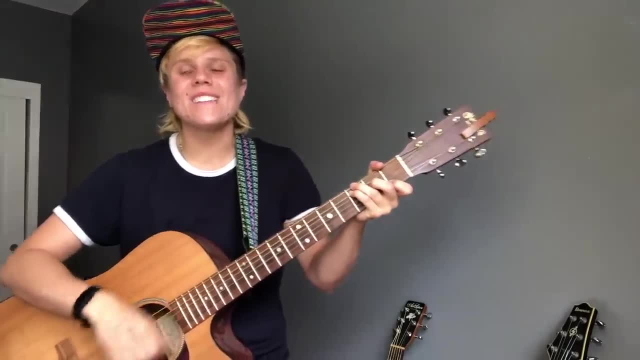 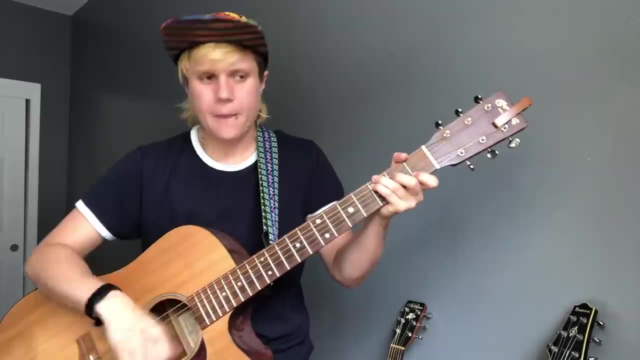 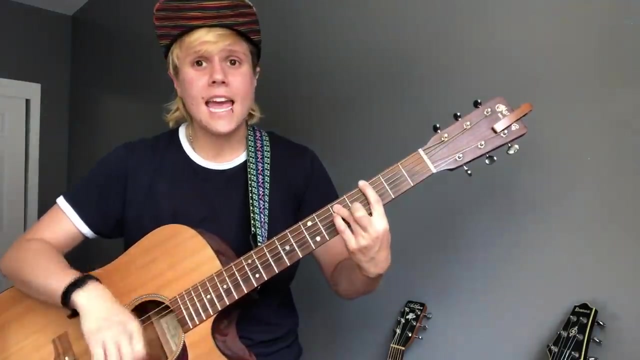 One, two, three rocking guitars. One more time: One, two, three rocking guitars. One, two, three rocking guitars. Play all day, play all night. rock my way to a lullaby, Rock my way to a lullaby. 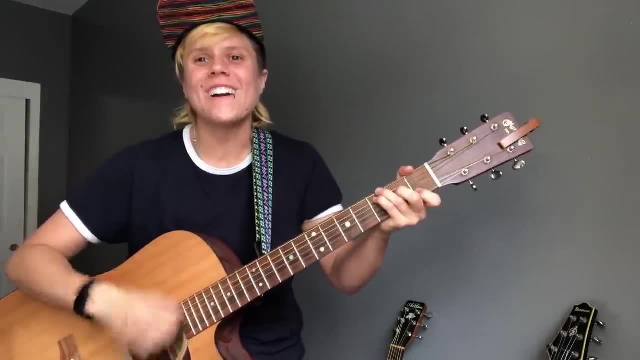 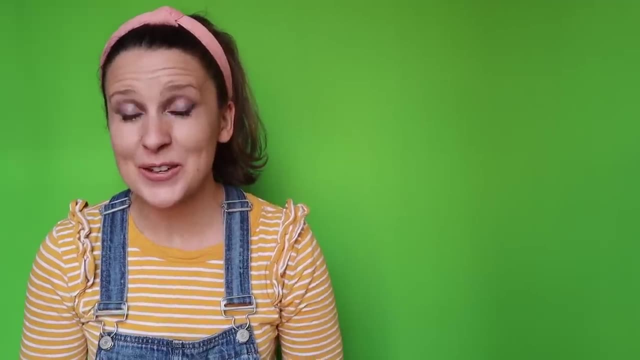 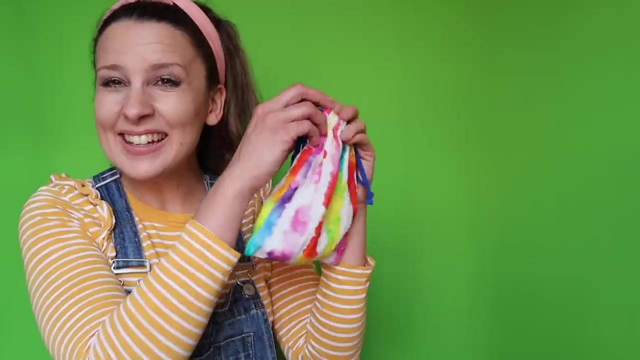 One, two, three rocking guitars. Thanks for helping me count my guitars and singing with me. I have something special to show you. It's in this little bag. Let's open it. Can you say open, Open, open the bag. 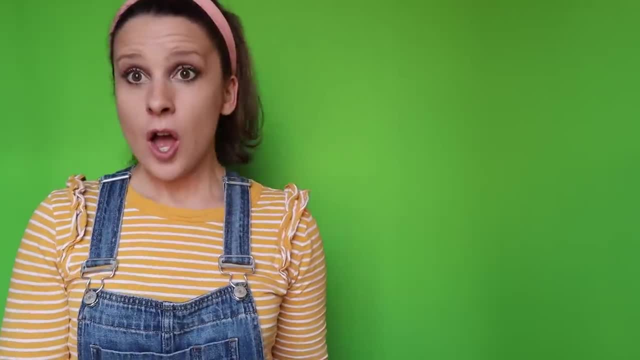 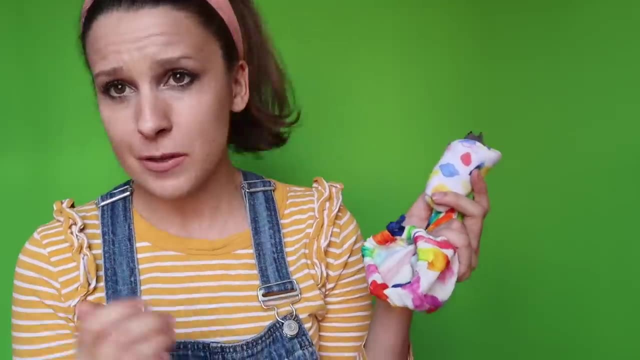 Let's see what's inside. It's a mouse. Oh shh, the mouse is sleeping, But it's time for the mouse to wake up. Let's say: wake up mouse. One, two, three, wake up mouse. 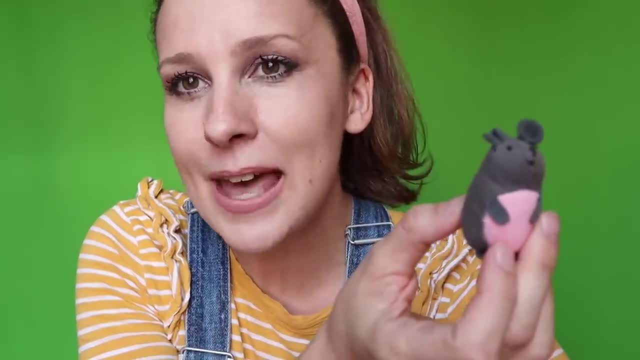 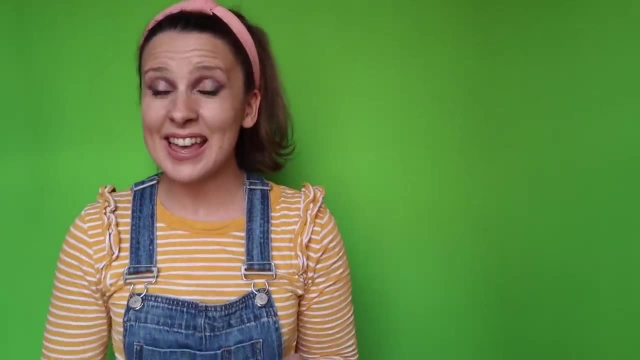 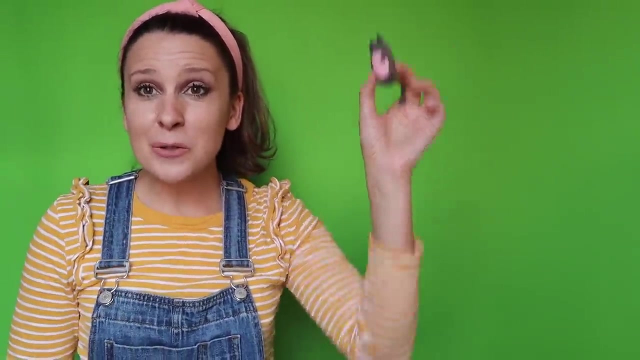 Oh, good morning Hi, I'm a little mouse, I want to climb up the clock. Can you sing Hickory Dickory Dock? Sure, we can sing that Hickory dickory dock. The mouse went up the clock. The clock struck one. the mouse went down. 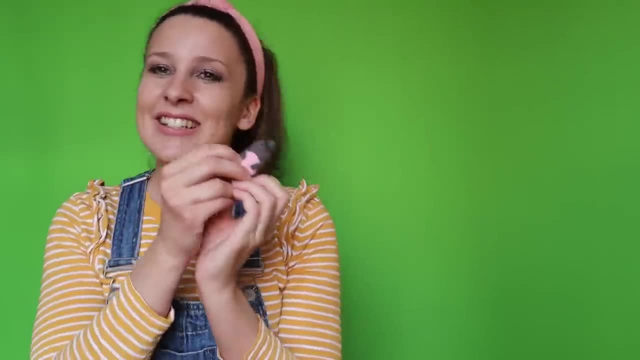 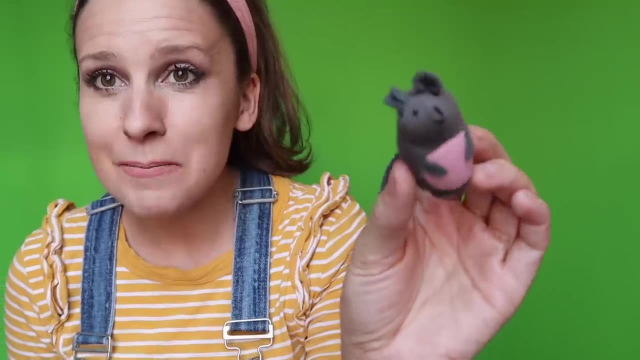 Hickory dickory dock. Tick tock, tick tock, tick tock. Hickory dickory dock. That was so much fun. Thank you for singing my song. I'm going to go back to sleep now. Good night. Oh shh, the mouse wants to go back to sleep. 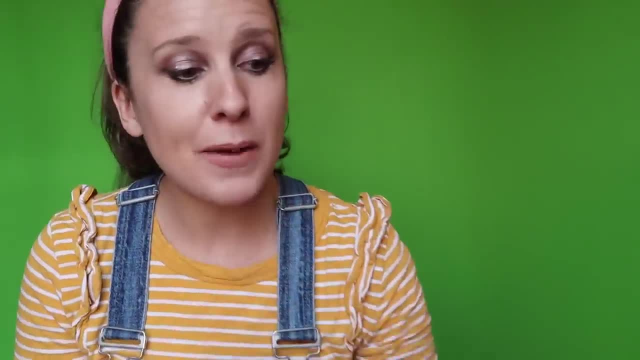 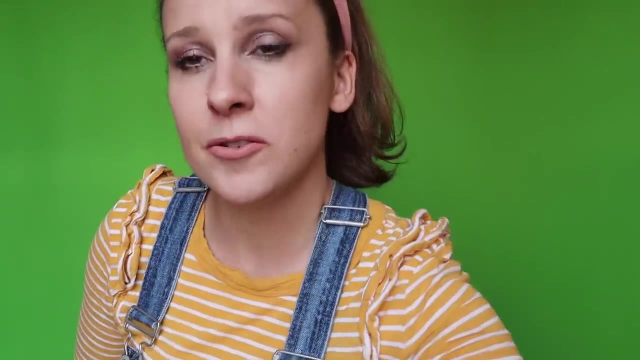 Let's whisper. Okay, let's put the mouse back in the little bag. Good night mouse Say, good night mouse Shh. I want to show you another song I know about a quiet mouse. Can you pretend your little thumb is a mouse? 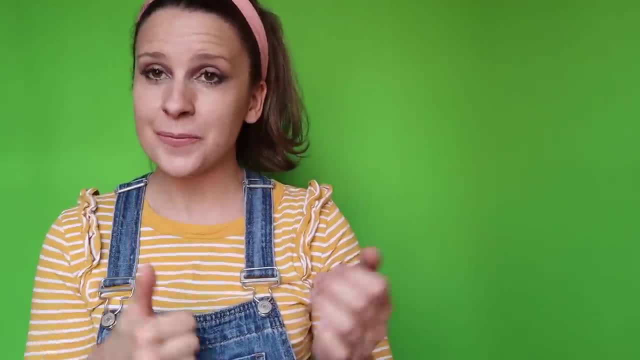 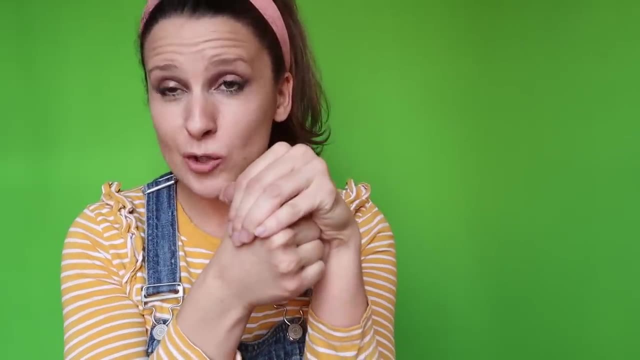 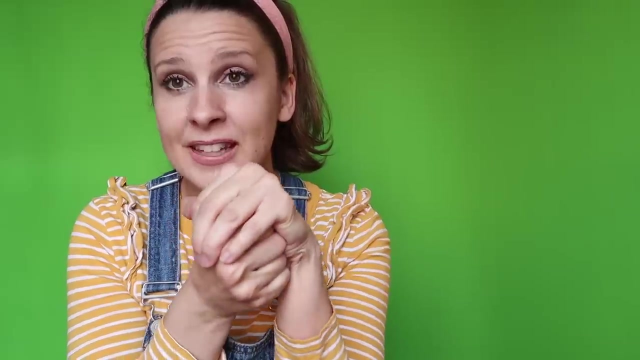 Then your other hand is going to be the house, A quiet little mouse in a quiet little house, When all was quiet as quiet can be. Shh, shh, shh, Alphatea. What a silly mouse. Let's try that again. That was so silly. 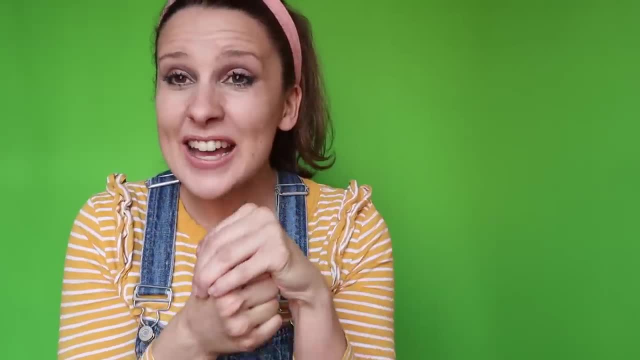 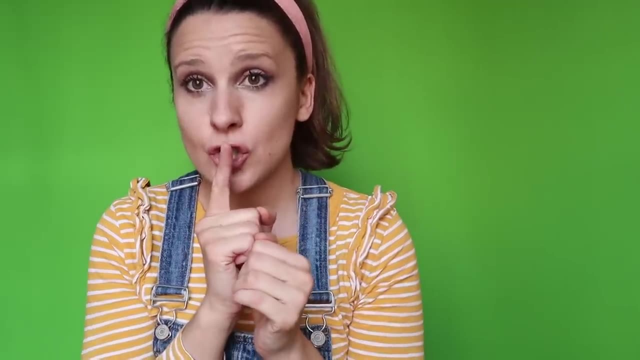 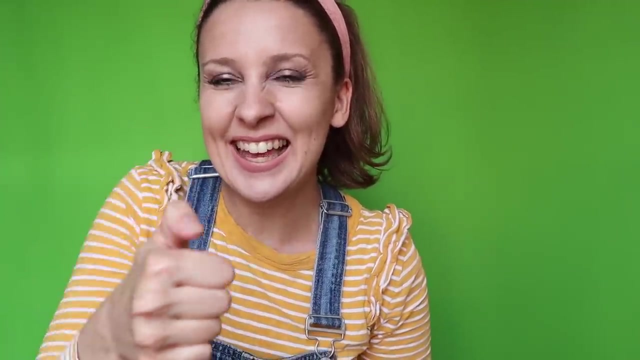 A quiet little mouse in a quiet little house, When all was quiet, as quiet can be. Shh shh, shh, Alphatea, That was so silly. The little mouse surprised us. Good job, Hey, everyone. 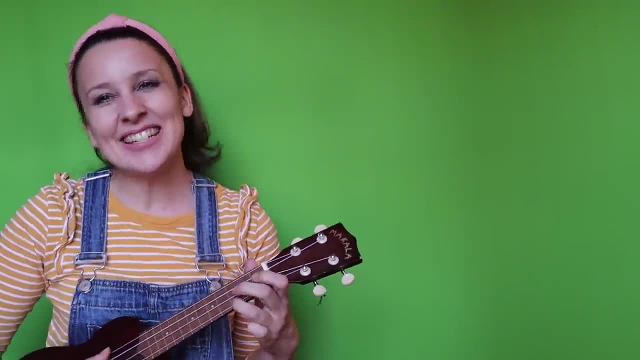 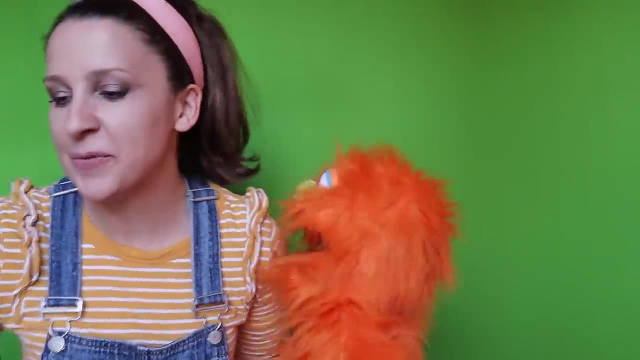 Guess what it's time for. Instrument of the Day: Yay, that's my other favorite part. Hi, Rachel, Hi, it's good to see you. Good to see you. The instrument of the day is the recorder. Wow, 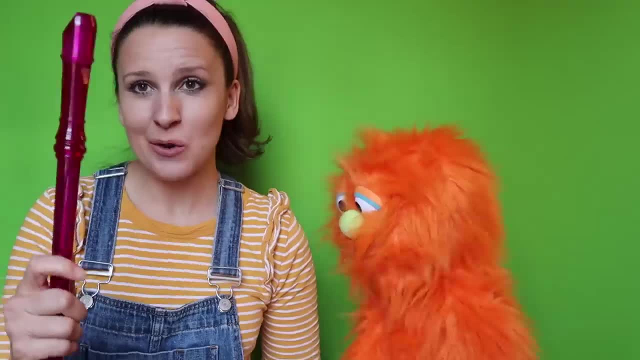 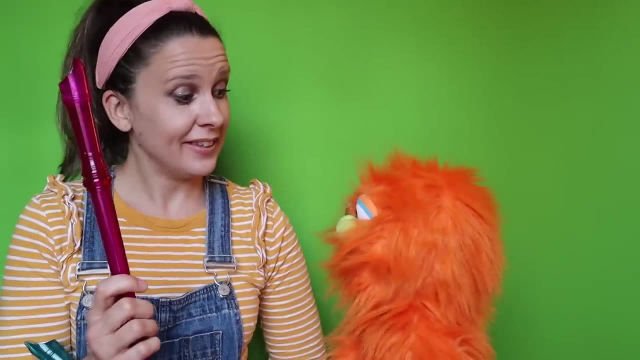 Let's see how many recorders I have Count with me. Okay, One, One, Two, Two. Yeah, Yeah, I did it. What color is this one? Fuchsia, Yeah, or we could just call it pink. 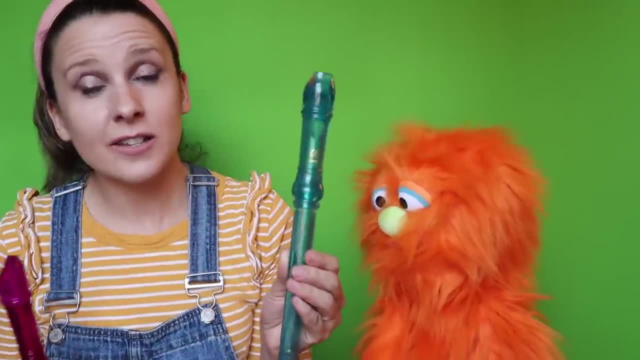 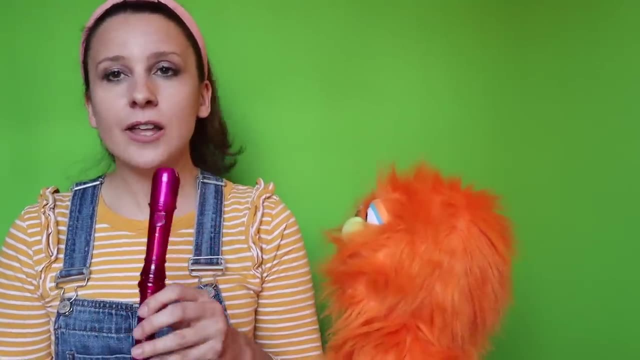 Pink. That's very specific. I like that. What color is this one? Blue, Yeah, great job, Blue. Do you want to hear how it sounds? Yeah, You can tell me if it sounds high or low. Okay, Does that sound high or low? 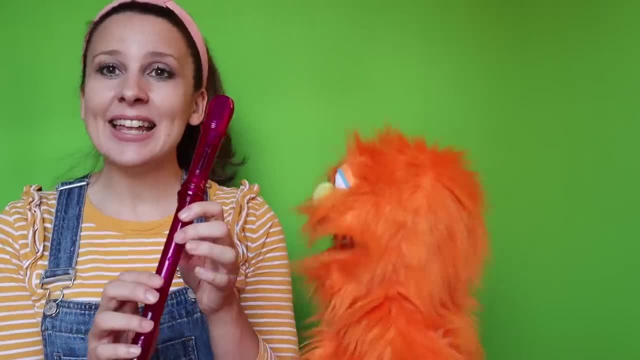 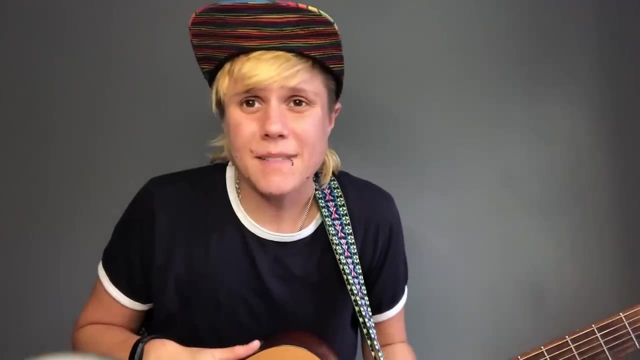 That sounds high. Yeah, it's high like a bird. It makes me want to dance on my tiptoes. Yeah, Dee, dee, dee, dee. Yeah, See you later. Hey guys, Sometimes I get really worried. 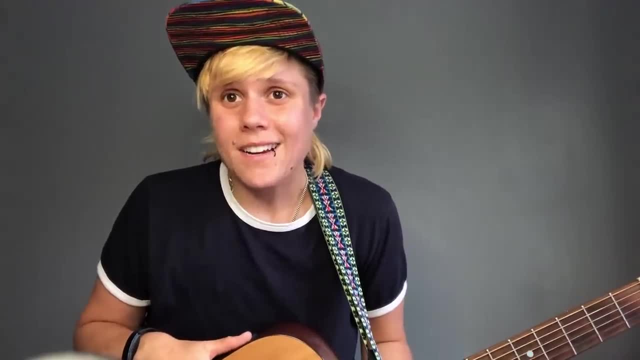 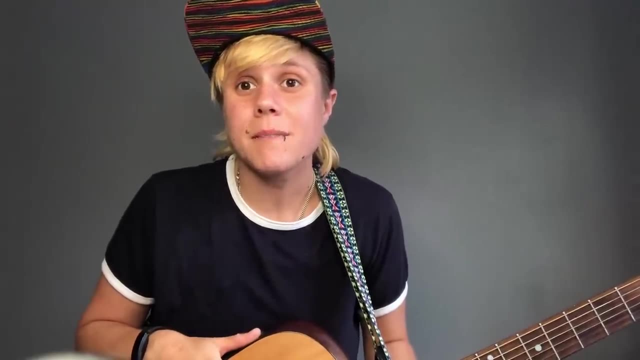 Whenever I don't know what's going on, I start to worry and get scared, and I put on music to help me calm down. I'm going to play you a song that I love. It's a song that I love that helps me not worry so much. 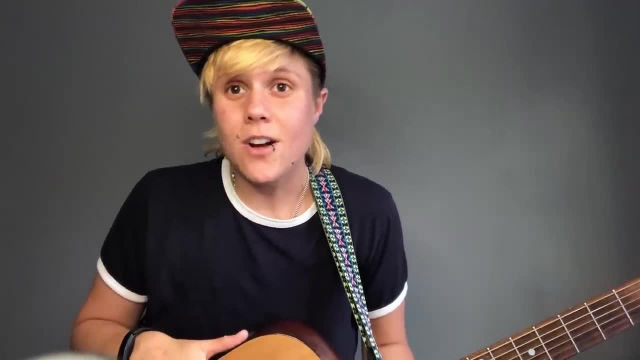 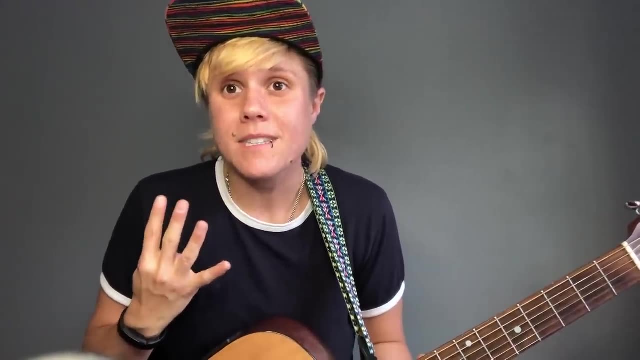 We're going to sing the chorus, which is the part of the song that happens more than one time. It happens one, two, three or even four times. That's a lot of times and that's how I know it's the chorus. 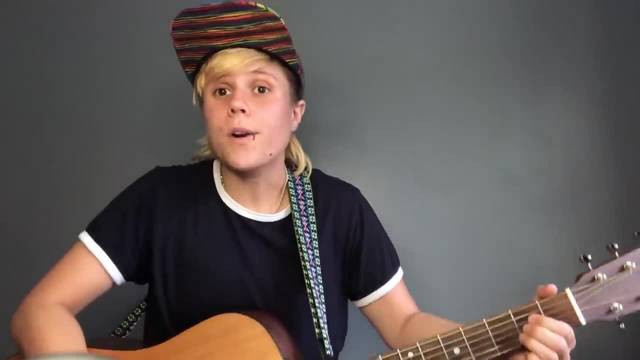 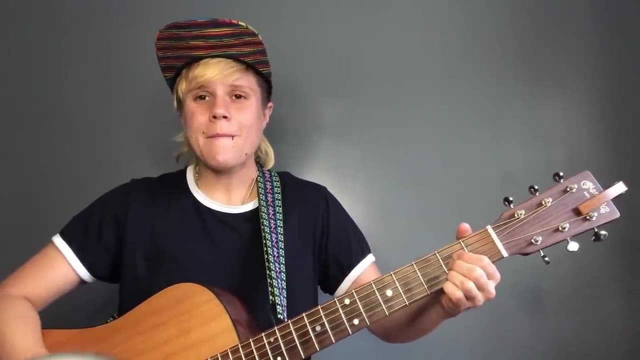 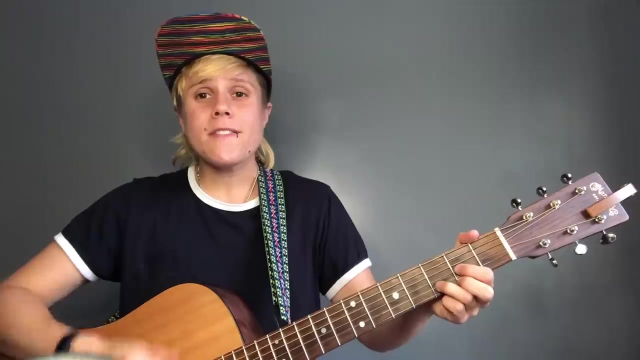 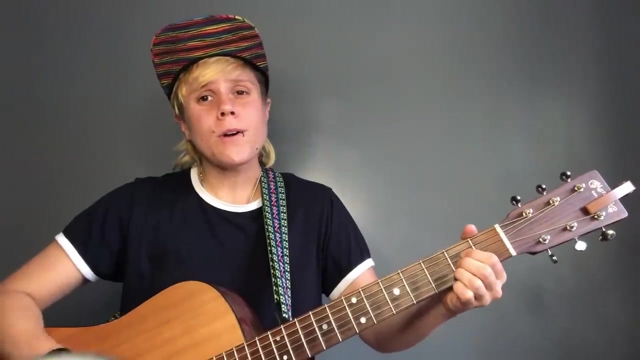 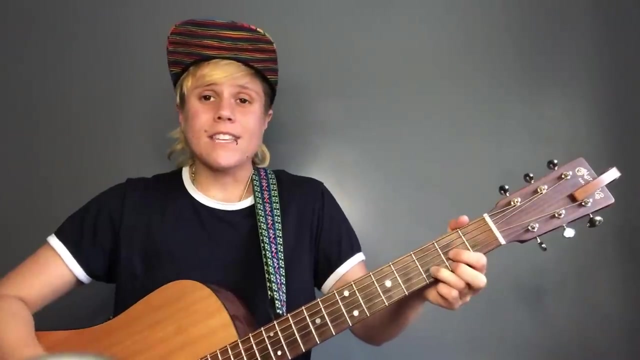 Are you ready? We're going to sing a song about not worrying. Don't worry about a thing, Because every little thing is going to be all right. Singing- don't worry about a thing, Because every little thing is going to be all right. 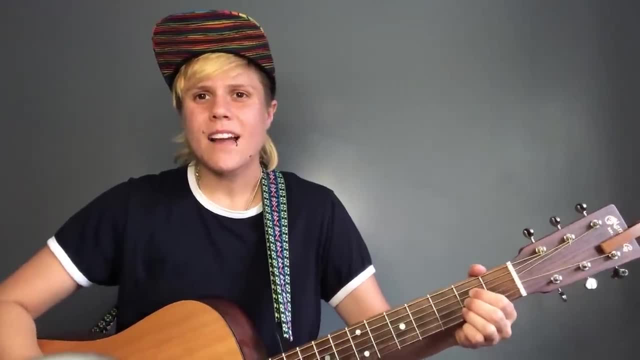 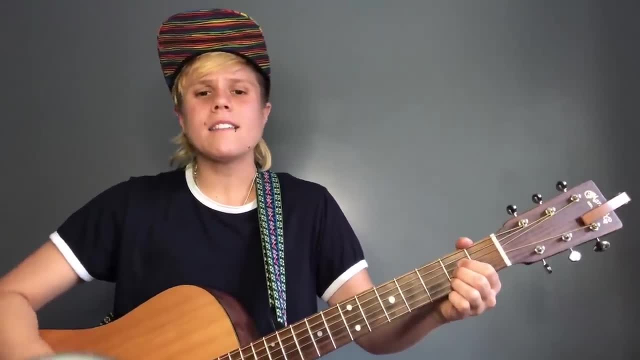 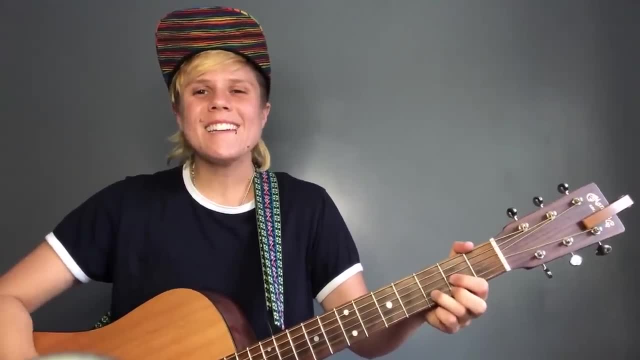 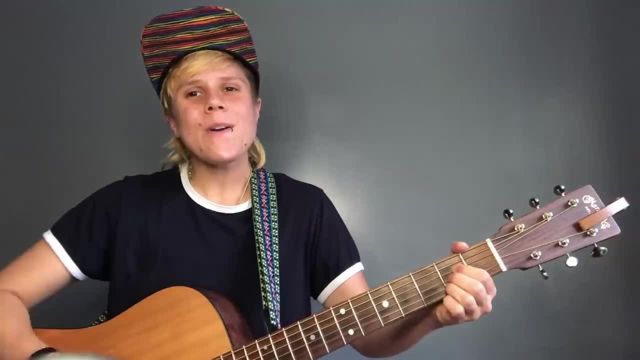 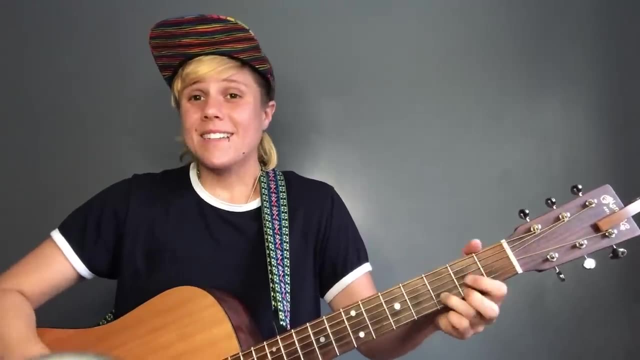 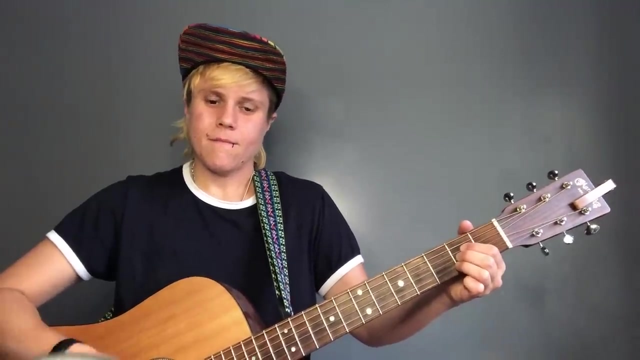 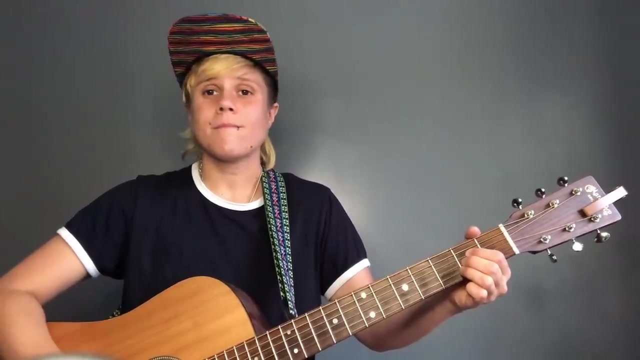 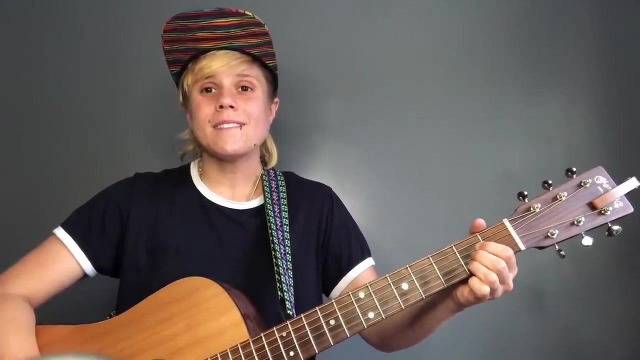 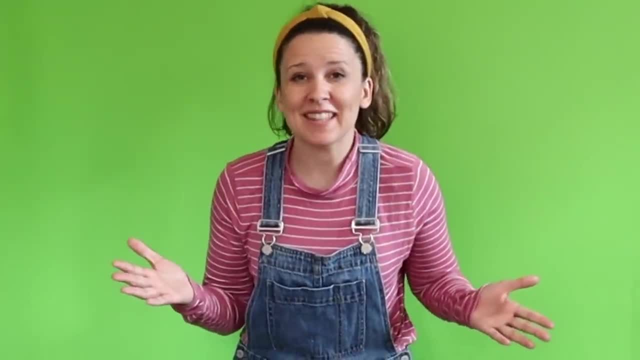 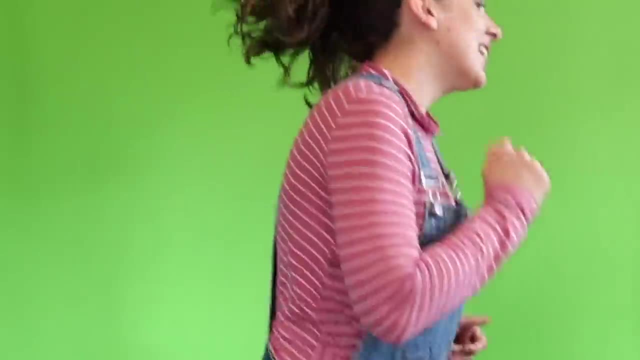 Let's take it back to Rachel. Do you know how to skip? Show me Loo loo. skip to my loo, Loo loo, skip to my loo, Loo loo, skip to my loo, Skip to my loo, my darling. 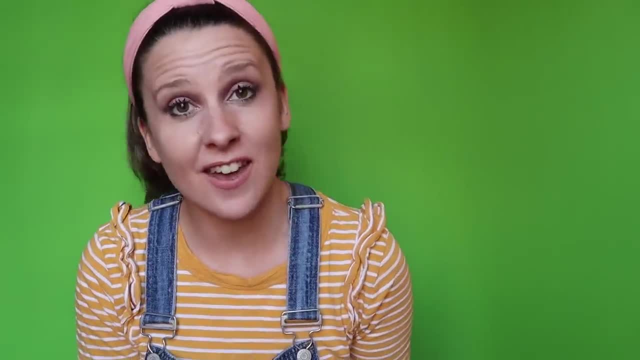 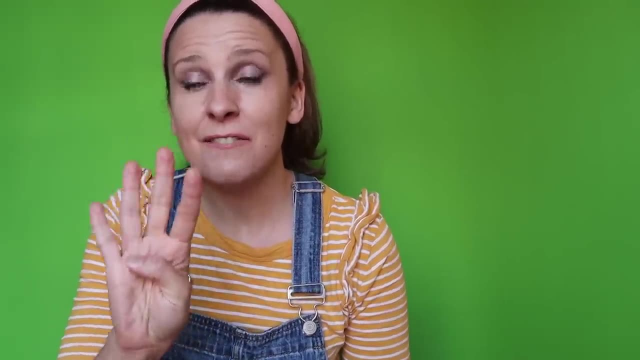 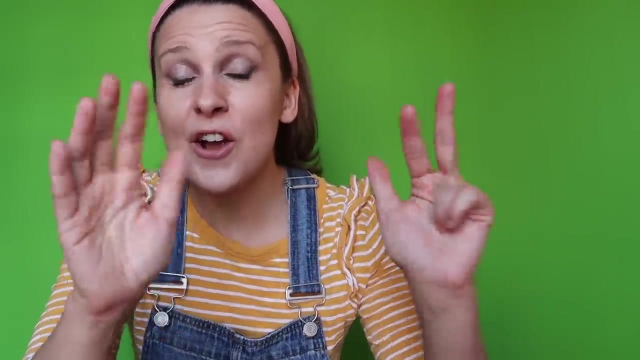 Great job. Do you know how many notes are in a scale? Let's sing a scale and see One, two, three, four, five, six, seven, eight. Wow, There are eight notes in a scale. Let's do it with the solfege. 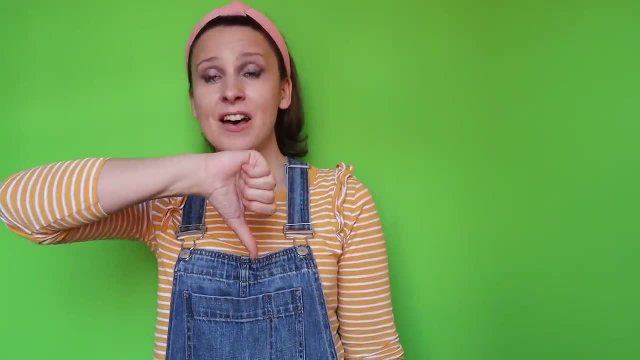 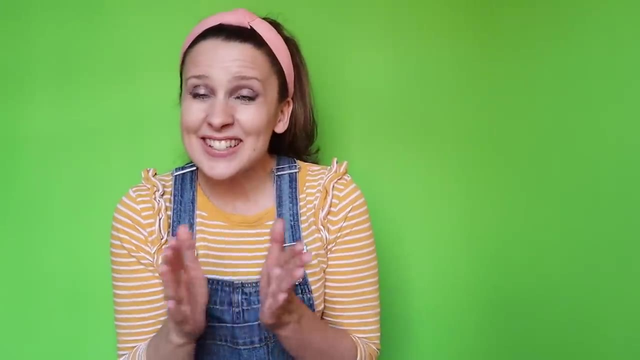 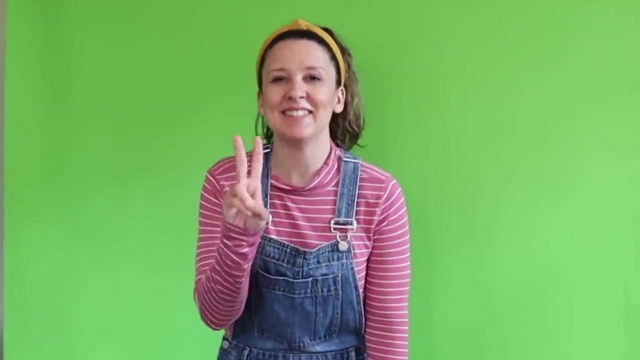 Do re mi fa so la ti do Great job singing your scale. There are eight notes in a scale. Can you jump when I sing pop One, two, three, pop Good jumping. One, two, three, four, five, six, seven, eight. 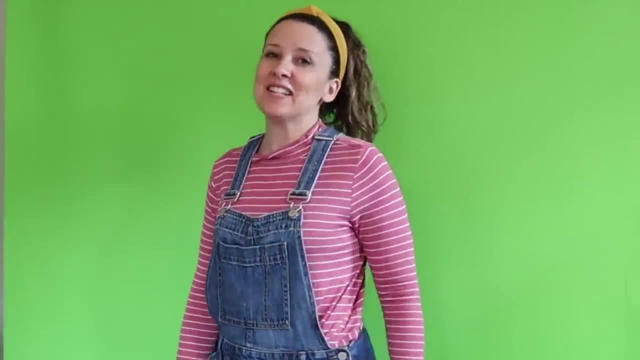 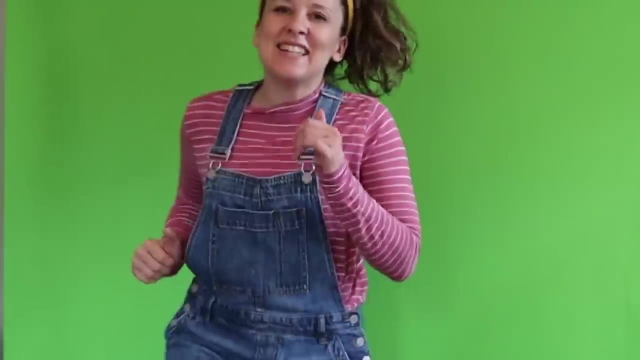 One, two, three, pop. Okay, now I'll sing, and when you hear pop, you jump. okay, All around the cobbler's bench. the monkey chased the weasel. The monkey thought it was all in fun. Pop goes the weasel. 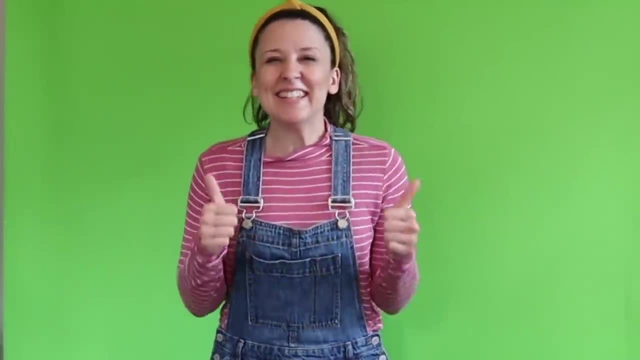 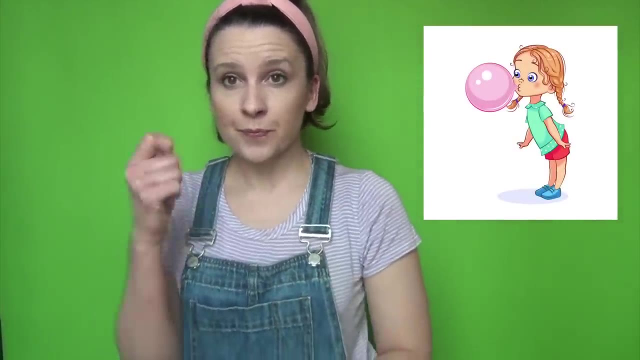 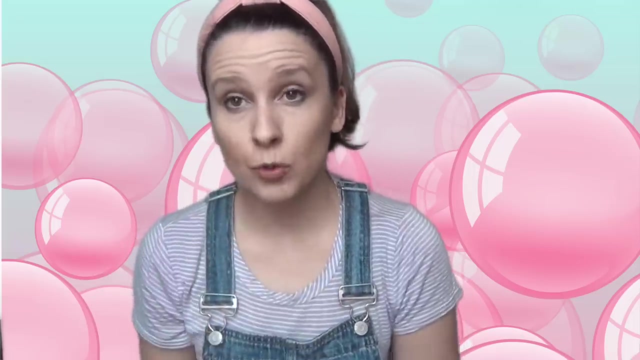 Yay, Did you jump when I said pop, Good job, We're going to get out some pretend bubblegum. Okay, so get out some pretend bubblegum. What color is yours? Mine's purple Pink. Put it in your mouth and we're going to chew it. 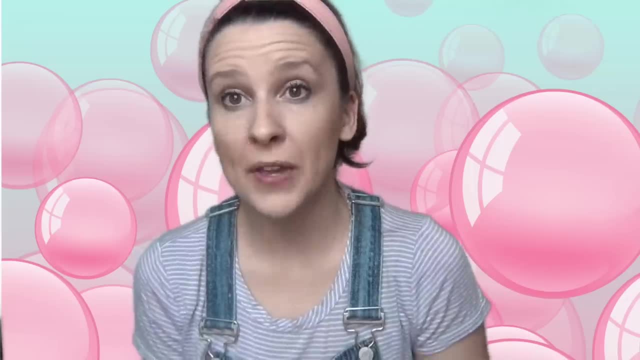 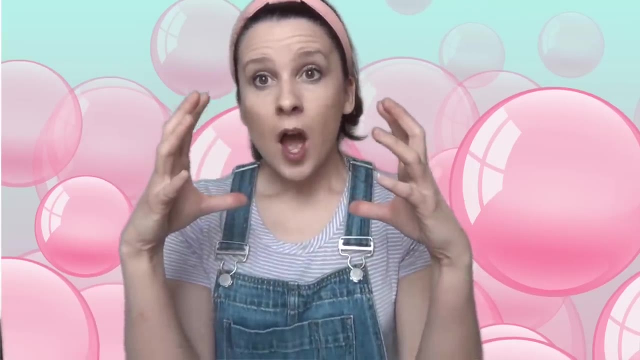 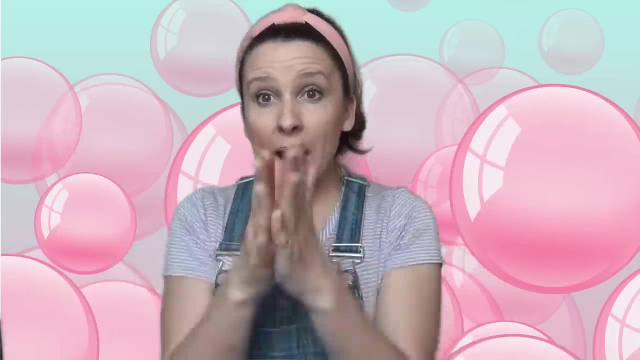 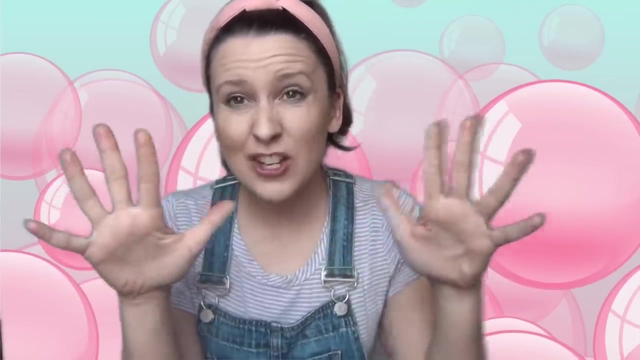 Are you chewing your gum? Okay, now we're going to blow a really big bubble. Are you ready, Ready? Wow, Pop, Oh no, Our bubble popped And the sticky bubblegum is all over the place. It's all over our hands. 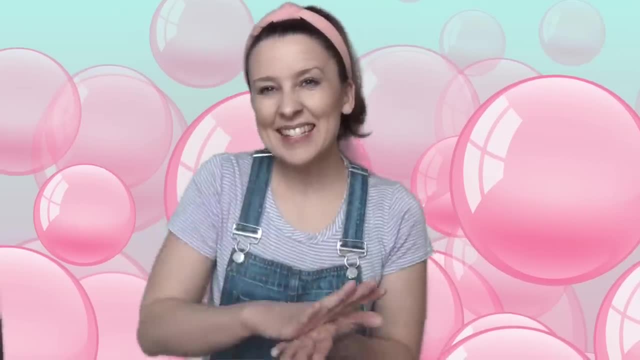 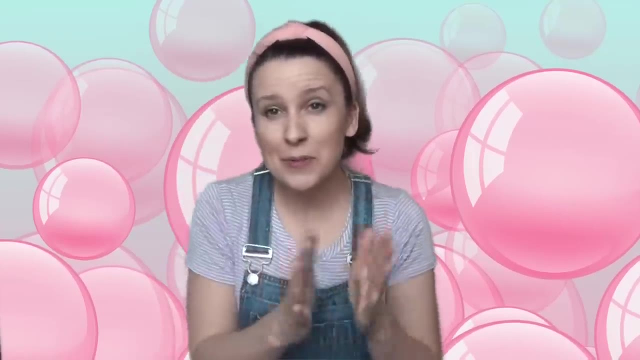 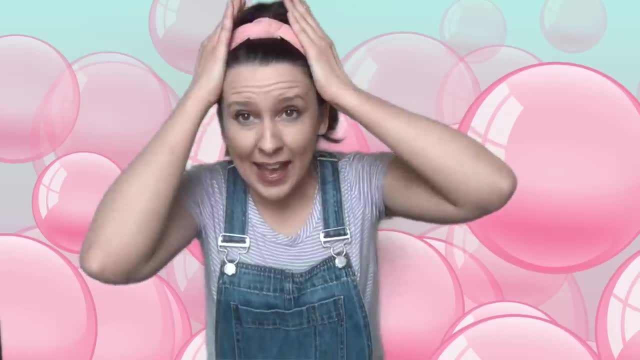 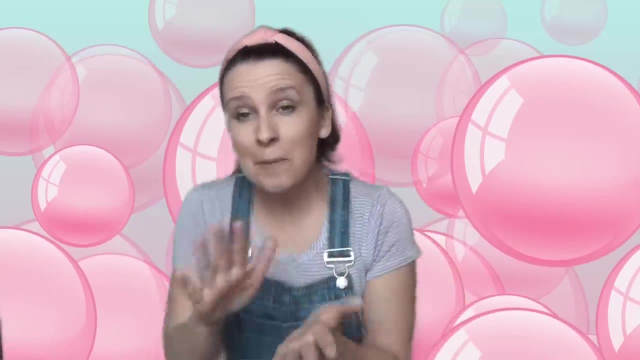 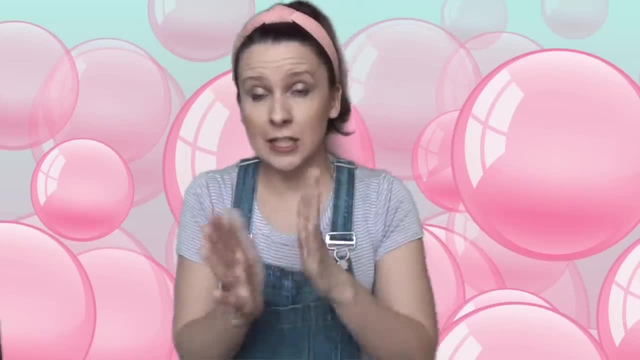 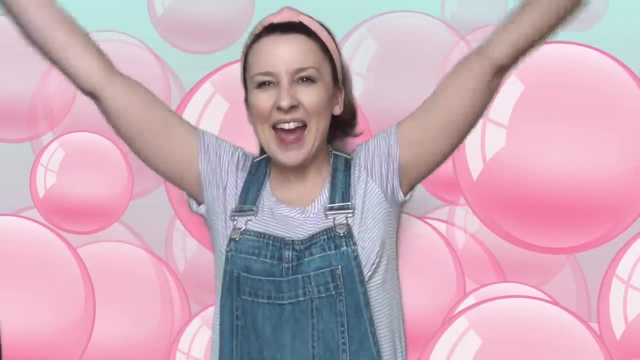 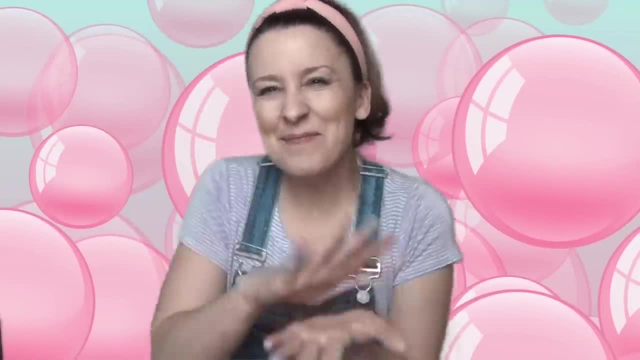 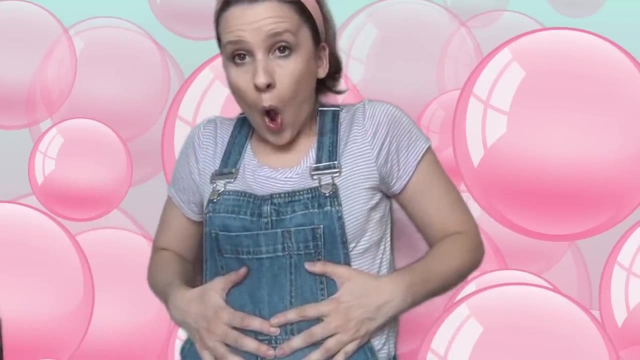 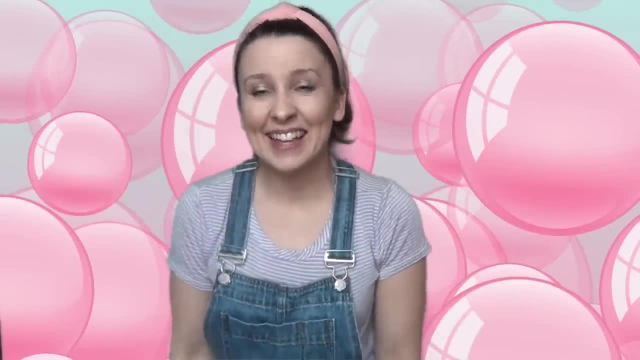 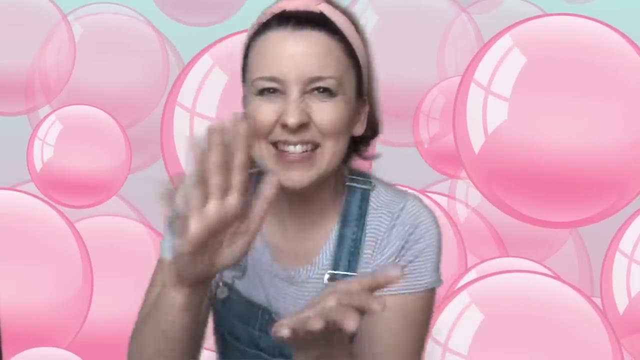 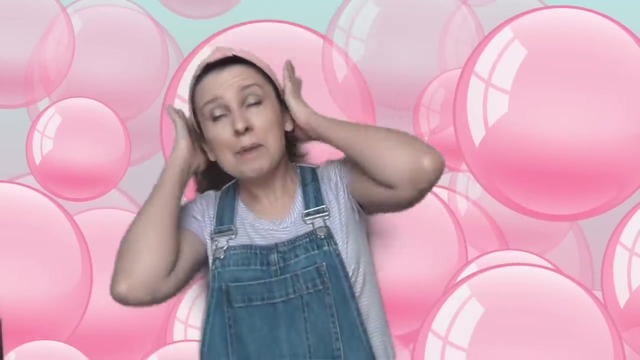 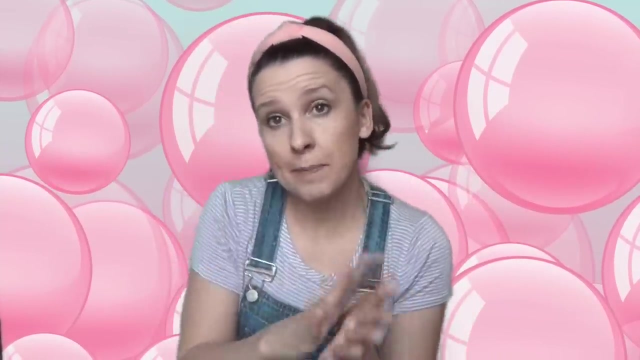 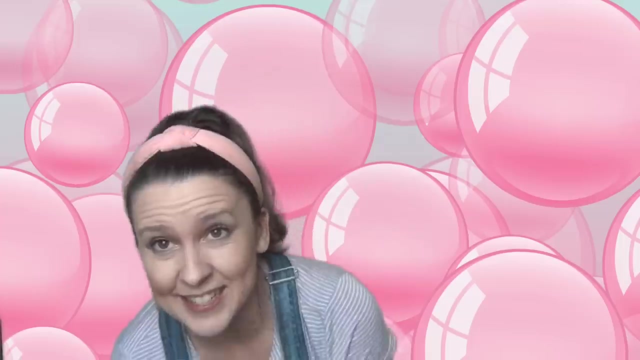 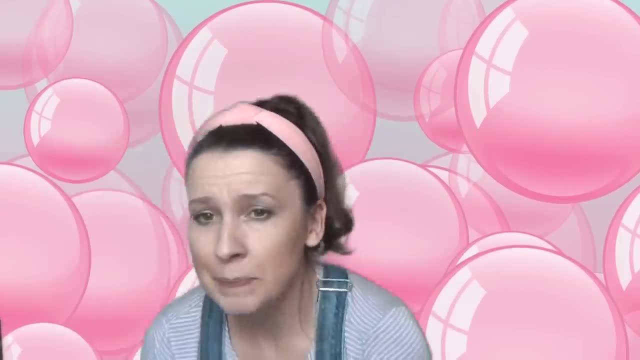 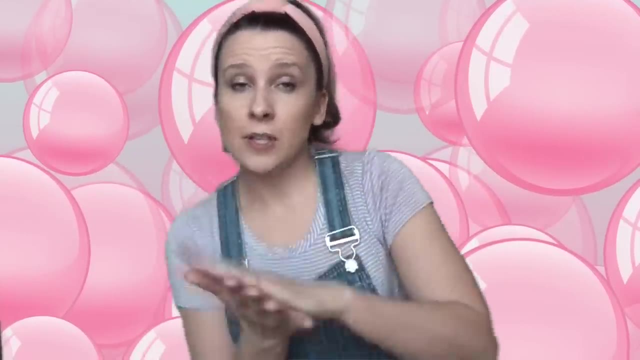 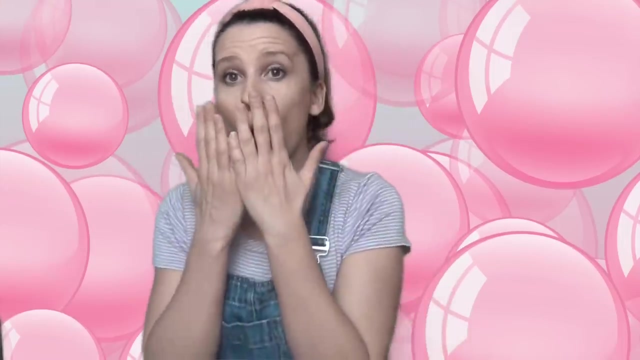 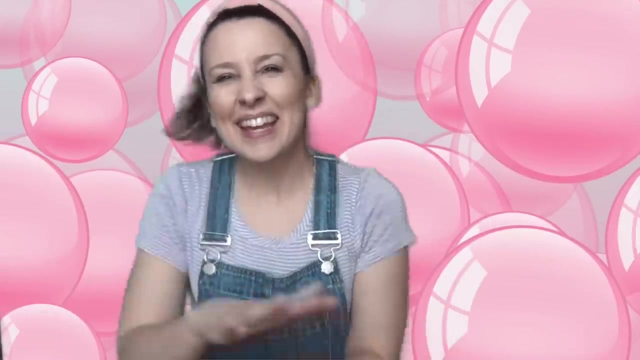 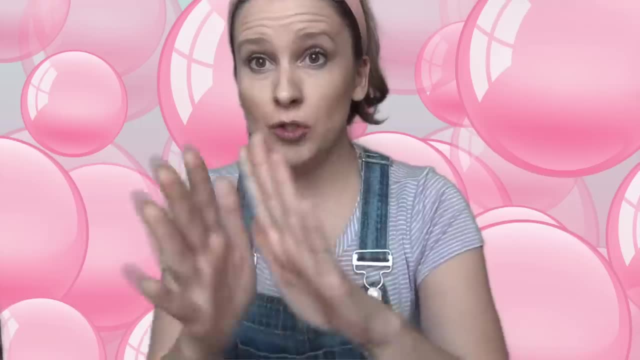 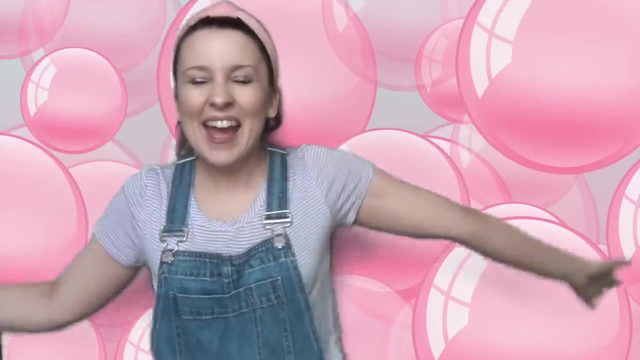 Icky, sicky, sicky, sicky bubblegum makes your hands stick to your grown-up. Put them on your grown-up And you pull them, and you pull them, and you pull them away. That was so fun. 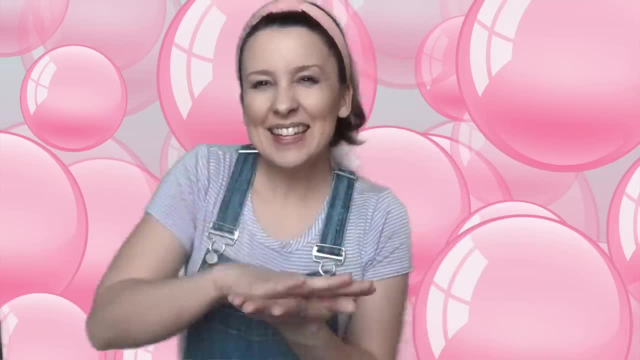 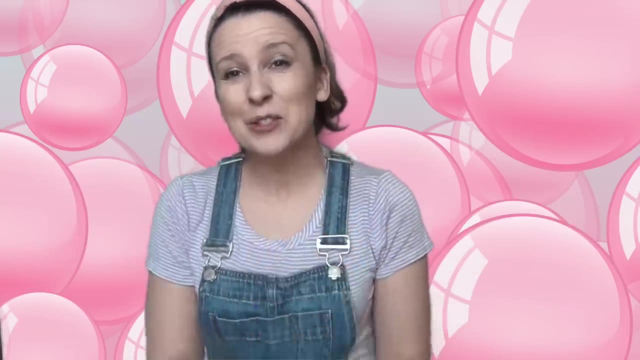 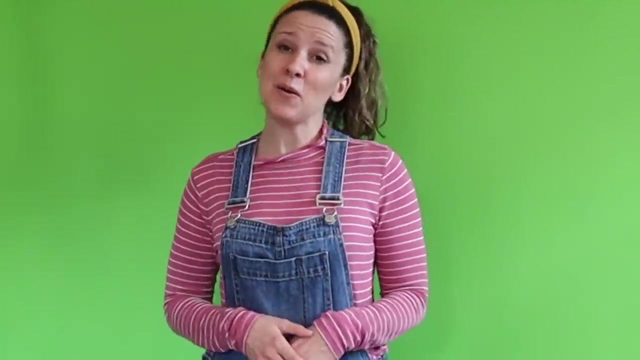 One more time. Icky, sicky, sicky, sicky. bubblegum makes your hands stick to your. Yay, That was so much fun. I have an idea: Let's play patty cake together, Or you can play it with someone at home. 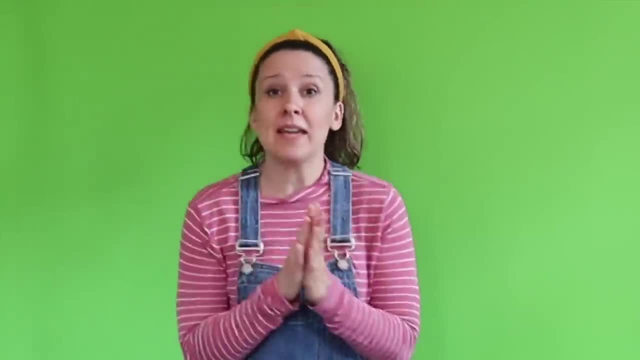 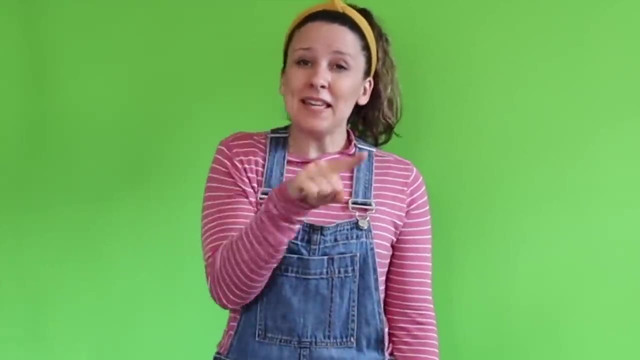 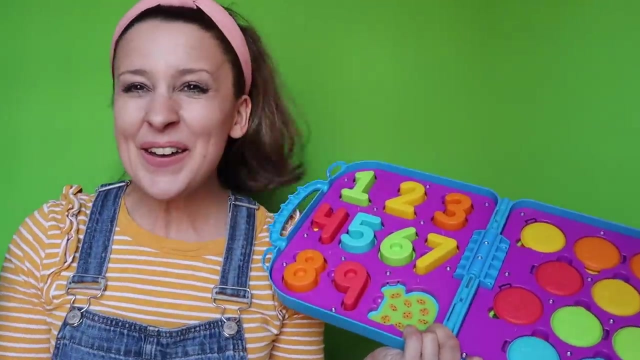 Patty cake. patty cake, baker's man, Bake me a cake as fast as you can. Pat it, roll it, mark it with a, B And put it in the oven for baby and me. Yay, Woo-hoo. 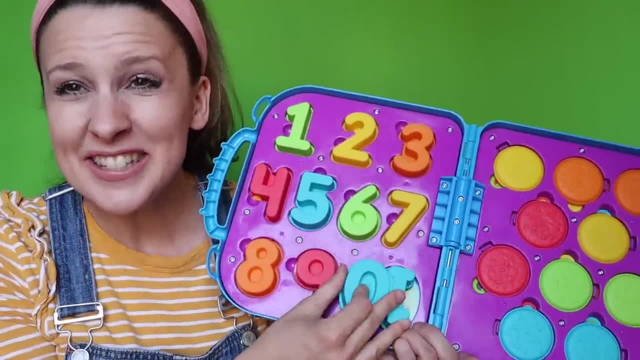 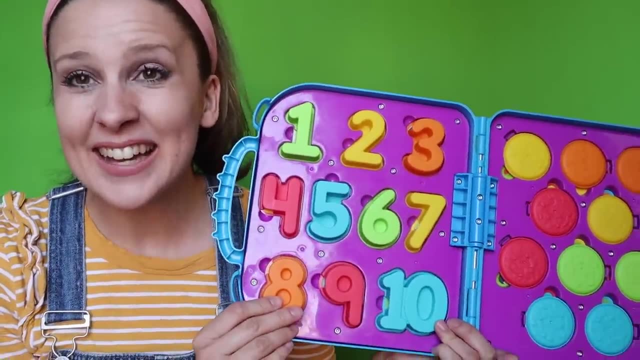 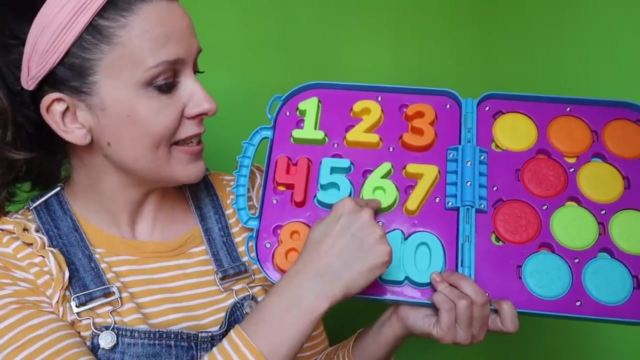 We sang so many wonderful number songs. The number 10 came back. Oops, it's upside down. Let's push it in. All our numbers came back. Let's count together: 1, 2,, 3,, 4,, 5, 6,, 7,, 8,, 9,, 10..